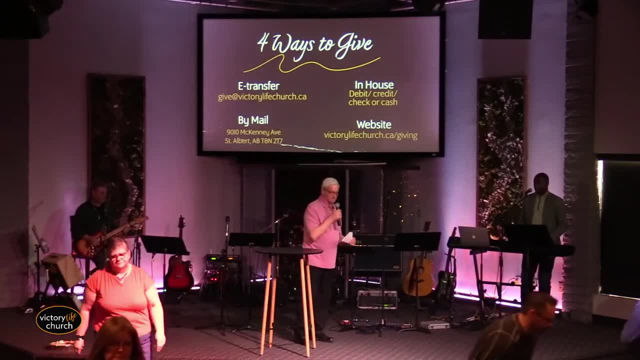 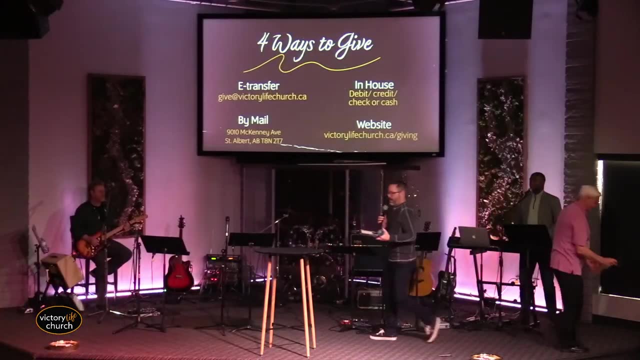 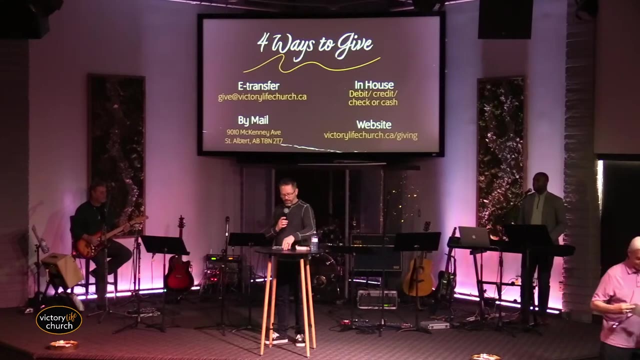 Thank you very much. God bless you as you give as well. Thank you, Pastor, Jerry. Well, good morning again, everyone. Great to see everybody in the house of the Lord this morning. How many of you were able to make it out Friday night for the team from Asia? 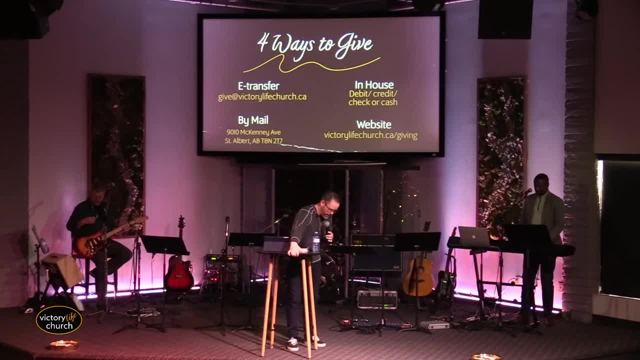 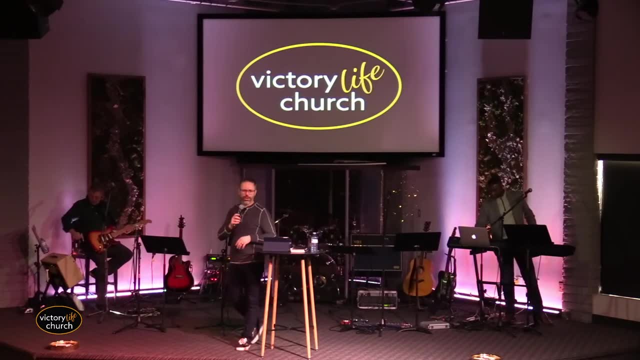 Wasn't that awesome, Wasn't that great that they came and they shared and they poured out with us and had some prophetic words over Canada. They had some prophetic words over our church And I was like man, this was such a great evening. 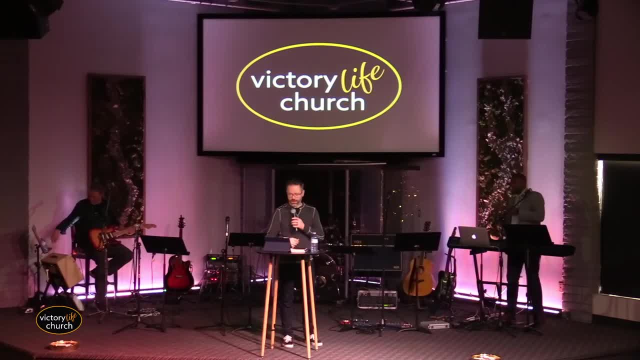 It was an awesome time And I just, Damien, one quick sec. Can you go check and see if all the- I think half of our stage lights aren't turned on here on the breaker, Because I'm like it's really dark up here and I feel like I'm standing in a shadow. 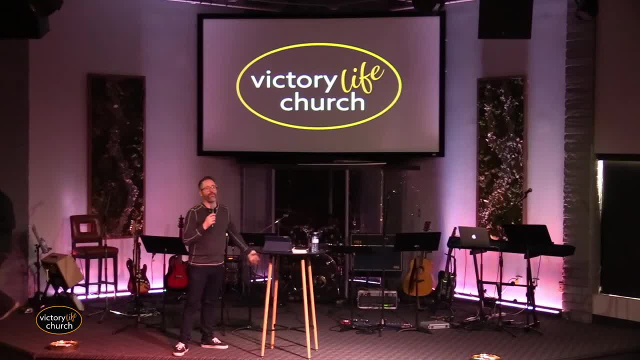 But our Asia team was awesome And they came. you know what? They came all the way over here on their own accord, on their own bill, on their own thing, And you know what? Today I want to bless them as a congregation, as a church body. 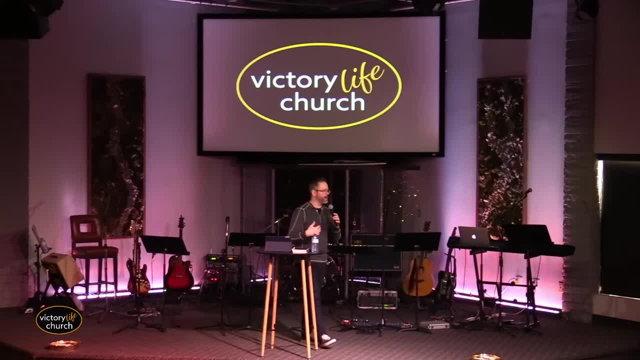 for pouring out into our church and choosing to come here and be a part. And we asked them: like, would you guys come here and just pour out for our team? And they said, yeah, we'll do it, We'll do it. 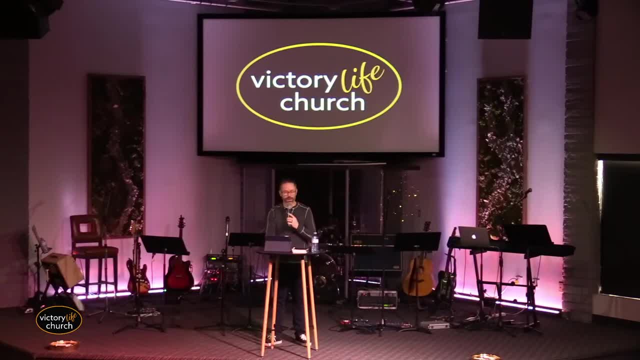 We'll do that. They're traveling around and doing all of this for nothing, with no expectation, And you know, I want to, as a church, as Victory Life Church, say thank you, You know what. So, if it's in your heart, this isn't a have to or whatever. 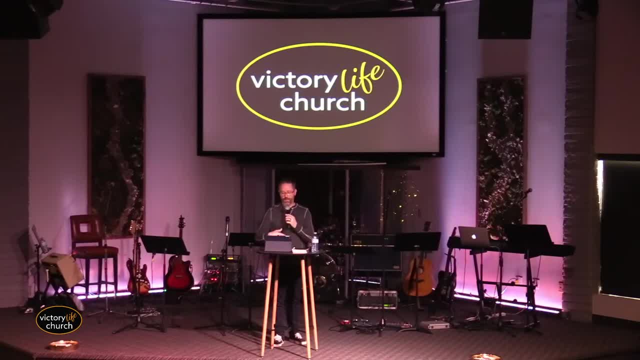 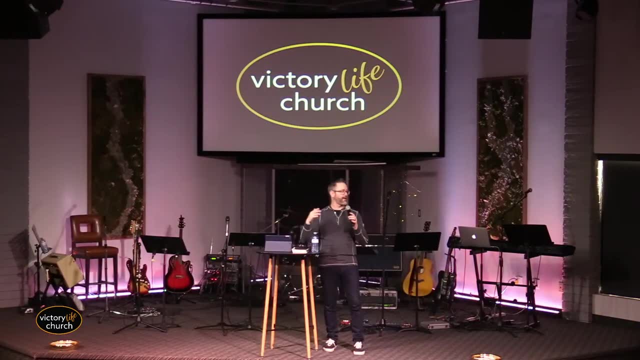 but if it's in your heart to give today, you know what? If you're watching online- and you watched it because I know there was like 1,300 views of it last night- Hey, there we are. There was 1,300 views of it. 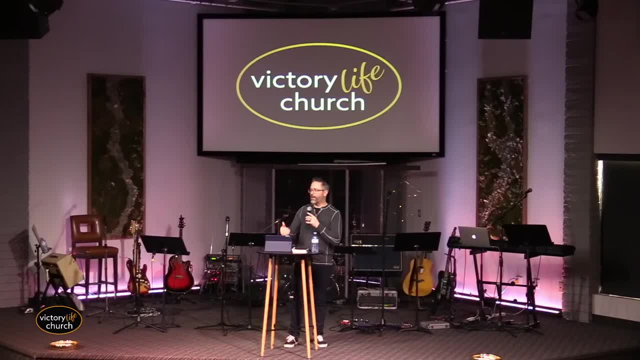 Just on yesterday morning of people watching from all over the world, I looked at the comments from Colombia and Asia and the United States and all over the place, And it was amazing to see God's word going out and touching hearts. And so if that's something you want to do, if you want to do it. 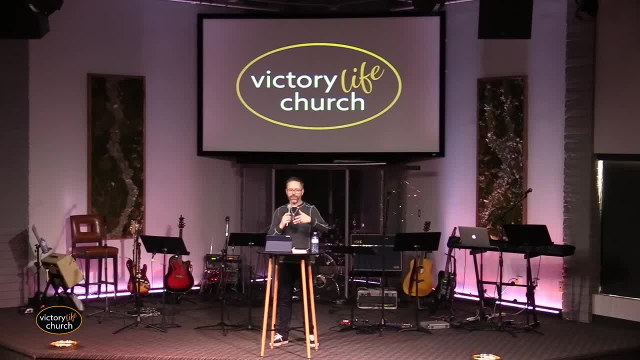 we can give in the exact same way as our normal giving- by e-transfer or PayPal or anything like that- But just market Asia team. If that's on your heart today or you want to do something at the Connect Center, just market Asia team. 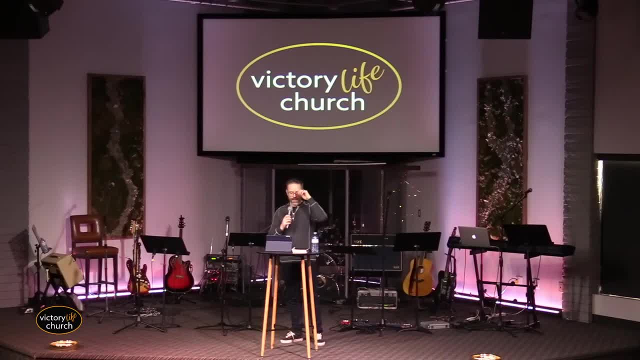 And we'll make sure that that That gets to them. But I just wanted to ask that of our church If there's anybody that wanted to do that. we didn't ask for it the other night because it's something I wanted to say. thank you as a church ourselves. 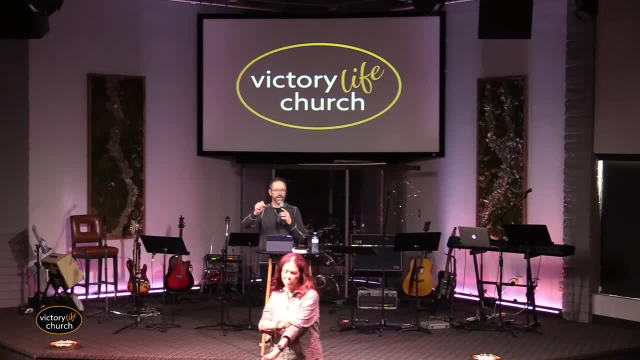 Again, if you're going to do that, just fill out an offering envelope: market designated Asia team. If you're doing it online, just put a note in it: Asia team- and we will make sure they get it. Amen, Okay. 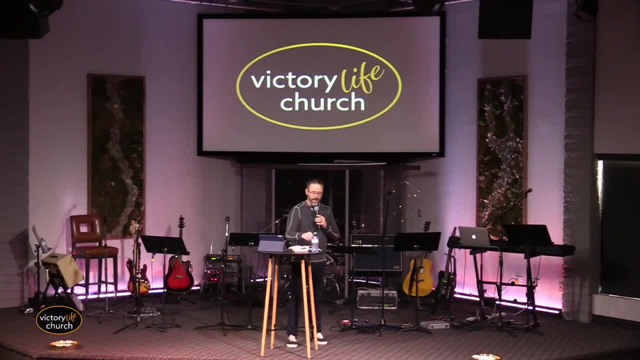 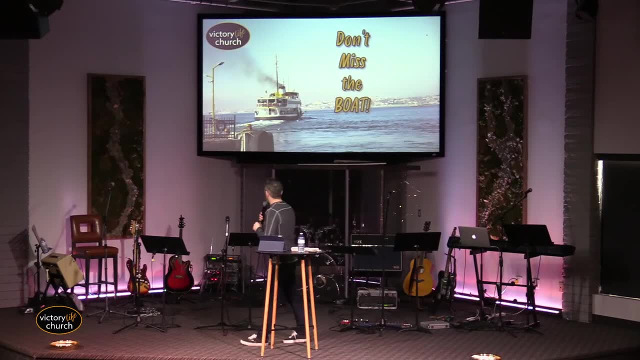 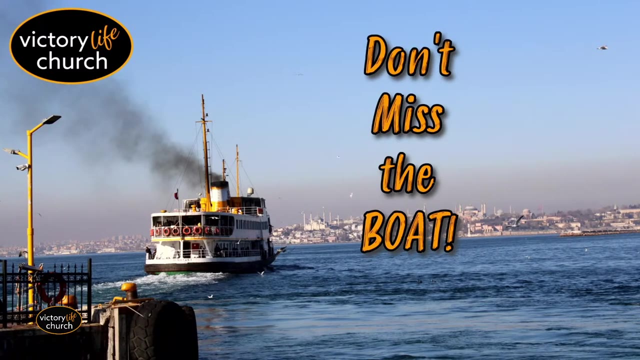 Let's see if we can get through this here this morning. Anybody here ever heard the saying don't miss the boat? Don't miss the boat. You're standing on the dock and the boat is taken off and it's gone, And usually we'll say that line. excuse me, 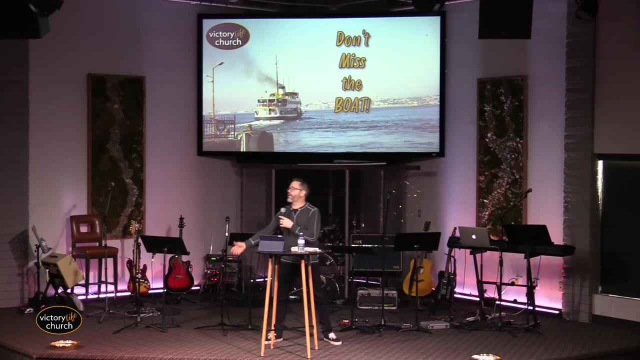 don't miss the boat on this opportunity, Don't miss the boat on this relationship, And we say that implying that, missing the boat, you'll miss out on reaching a destination that is blessing for you, Reaching a destination that has something good. 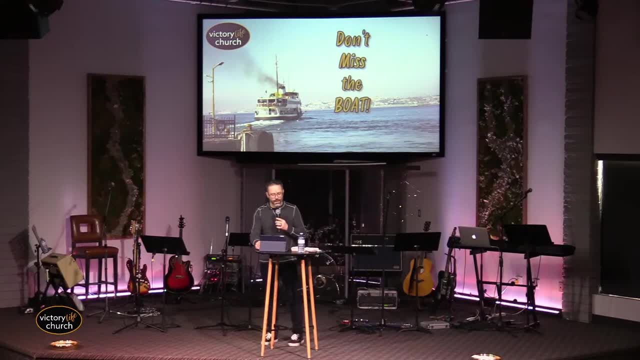 something great in store for you, And I've titled this series Don't Miss the Boat because I want to look at a few different things in the Bible that we can learn from being in the boat and being on the boat And what happens sometimes in the Bible. 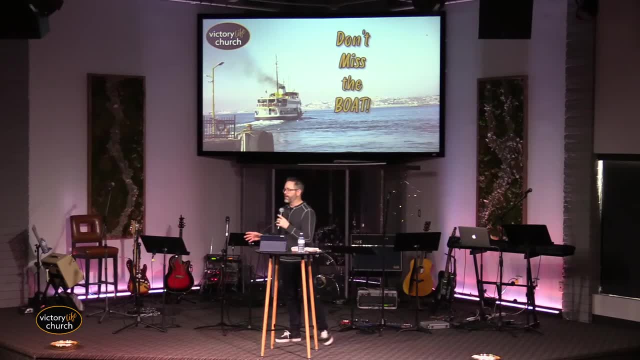 there's lots of recounts in the Bible of things that happened with boats And I took some time to spend and looked at a few of them and it was like man, there's some things we can learn Why we don't want to miss the boat, amen. 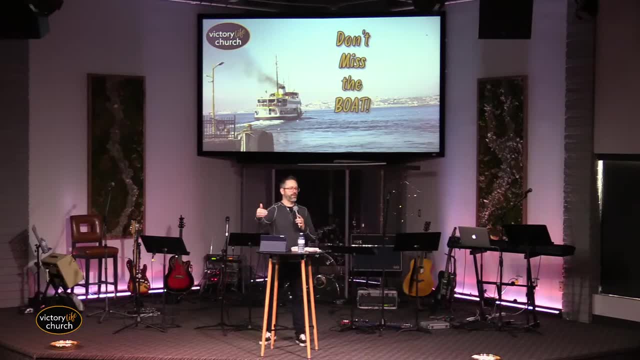 Because we want to learn what can lead us to greater things. Anybody here not want that? Anybody here not want greater things, Didn't think so. We want greater blessing and expansion as families, as individuals. amen, Okay, quiet bunch this morning. 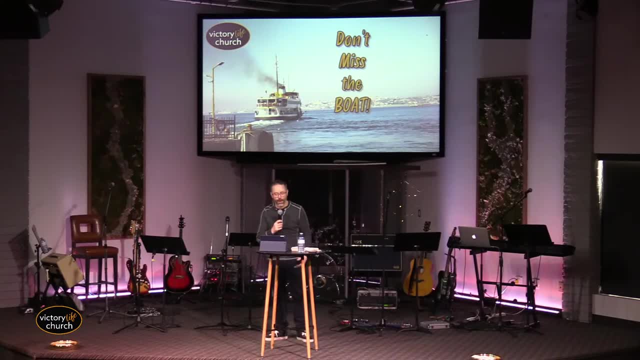 We want expansion and greater things. as a church body, We want expansion and greater things as we set our hearts to the mission of reaching those in St Albert who have not yet responded to the gospel, to the good news of Jesus Christ. We want to arrive at the destination of God's plans and promises for us. 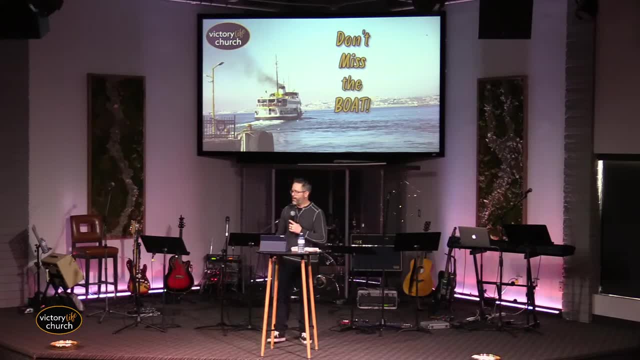 Don't miss the boat. Now I recognize sometimes we get on the boat and we think, oh, we're on the boat, now it's smooth sailing, Right. You get on the boat and you're thinking, okay, if you're going on holidays and you're getting on the road. 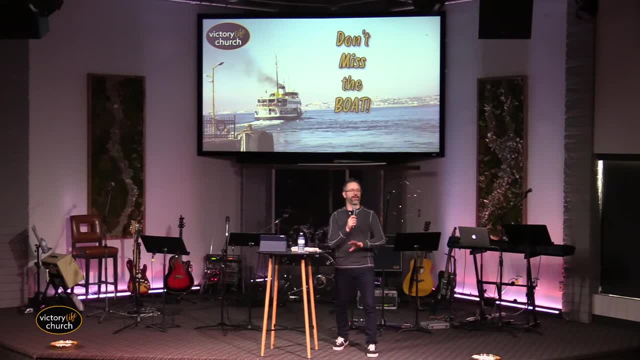 or you're getting on the plane, or you're at the airport, or whatever, and you're thinking, okay, now it's smooth sailing, right, You've left work, nobody can reach you anymore, and you're like, ah, we're on holidays. 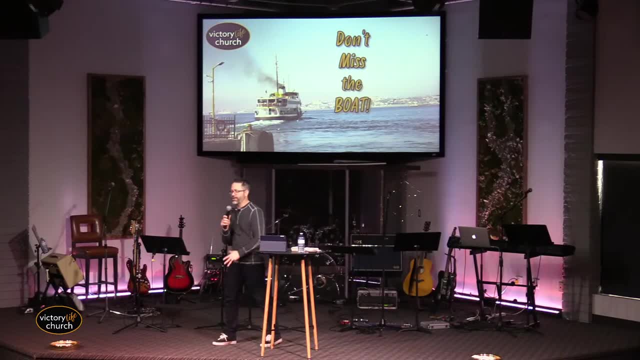 We're going to our destination, We're going to relaxation, We're going to restoration, We're going there. we're going there and a storm rolls in. Anybody but me ever had that happen. You're leaving, you get to the airport and you realize. 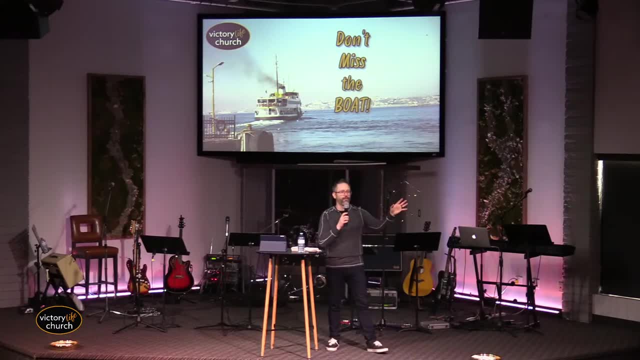 if Pastor Bob and Juanita were here, they could tell you the story of getting to the airport and realizing they left their luggage at home, Drove back home, got their luggage, got back to the airport and I think they missed their flight too, or something. 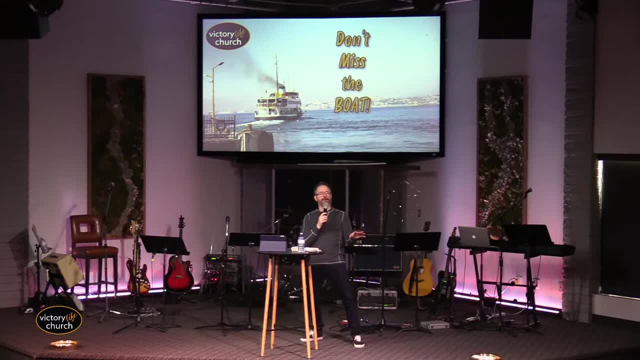 I mean talk about, you're just like, ah, we're here, We didn't grab the right luggage. Oh, my goodness, You get on the road. maybe you're a camper and you got your trailer hooked up and you're heading out and you're on the road. 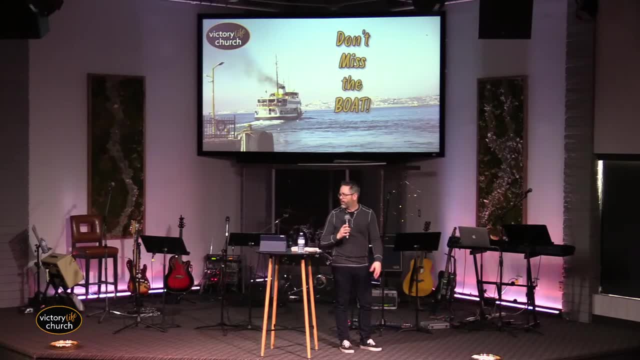 You get halfway out and you're like, ah, we forgot to get propane, or ah, you know, or something goes wrong with the truck or whatever, and all of a sudden a storm rolls in and for people on a boat with no land in sight. 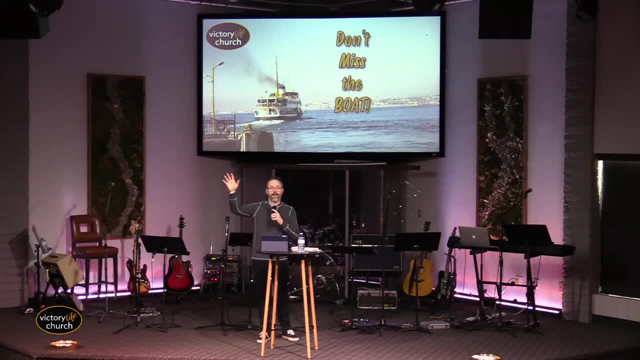 I don't know if any of you ever been on a ship out at sea or out and there's nothing but water around you and troubles roll in When you're in that place. I don't know about you, but storms are scary And sometimes when. 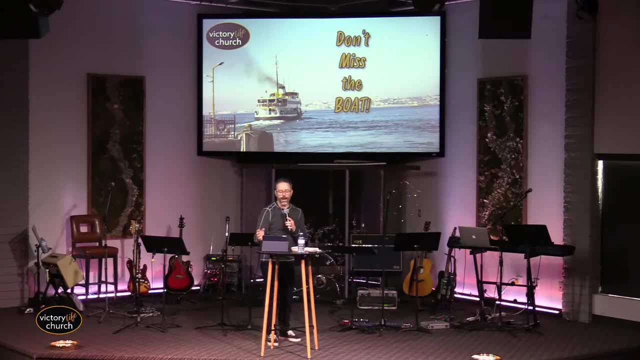 When storms arise in our lives, we feel like we're all alone, out at sea, miles from land, and we feel we have no clear direction and hope is far away. Amen, And isn't that the reality, right? The reality of some situations is we feel alone, we feel hopeless. 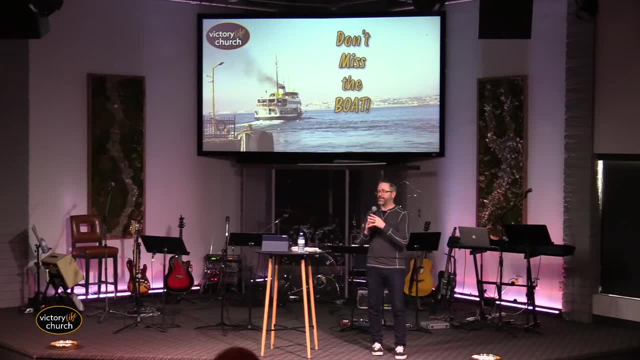 we feel lost. we feel like God. I can't see land anywhere, I can't see solid ground anywhere. What am I going to do? I'm going to sink here And it feels like all hope is lost. And this week's message I want to start in a place called the unsinkable ship. 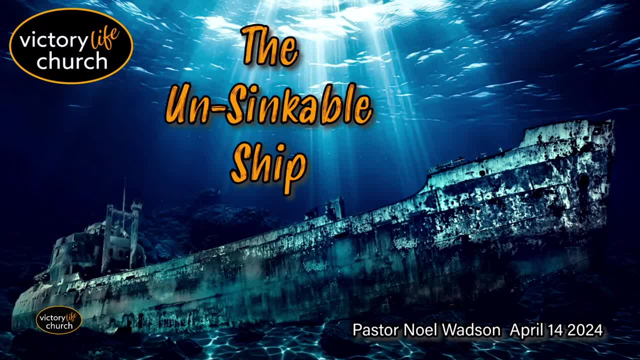 The unsinkable ship, Because you know what, Sometimes we set out for a destination I don't know. have you set out on a plan? You've got a plan for your life? You've got a plan for your future? You've got a plan for your business? 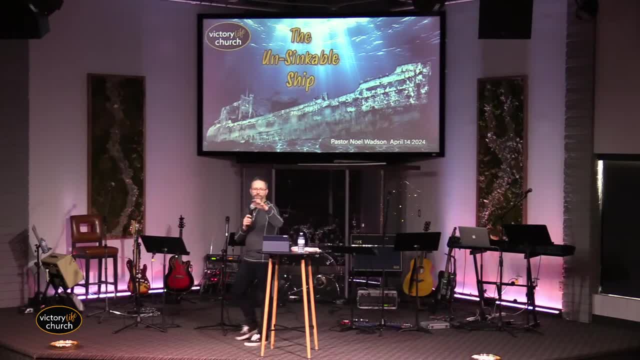 You've got a plan for your family, You've got a plan of some sort, You've got a plan for your schooling, And you set out And it seems like. It seems like your plans are unsinkable. I got it all together. 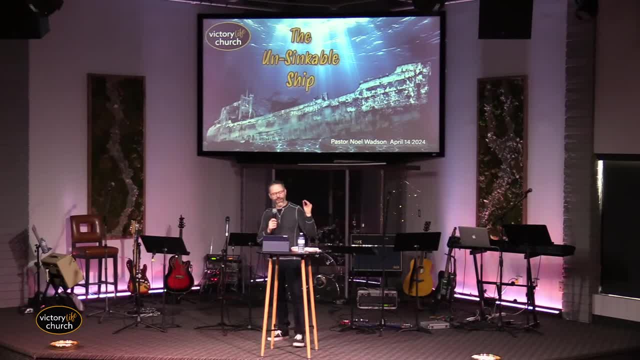 Is that just me? You seem like I got it all together, And yet the journey has led to pure chaos, trouble, problems, and it feels like everything's falling apart. Now, maybe it's just me and I get into that situation. 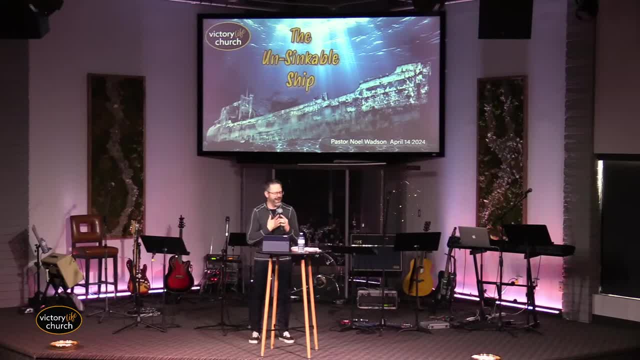 and I hear something inside and I know and I have said to somebody else or I've said to myself: man, that seemed like a good idea. That seemed like a good idea at the time. But I also remember when it seemed like a good idea at the time. 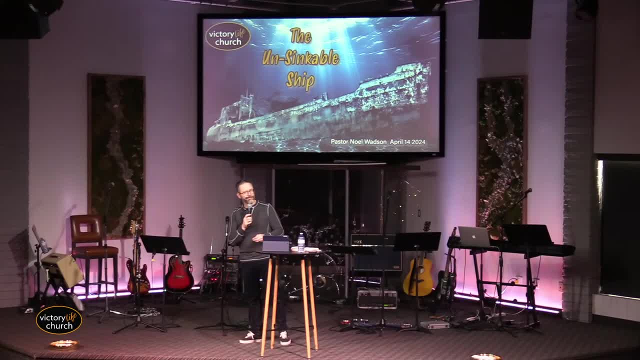 there was a still small voice inside that was saying, hmm, hmm, is it, though? Usually sounds like my wife's voice, But you'd have that small voice inside of you. You know, many of you here probably know the story of the Titanic. 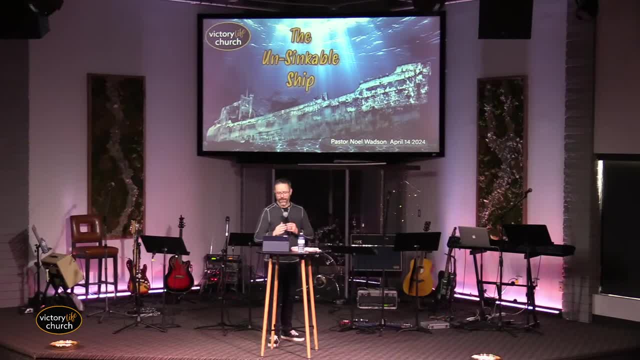 The unsinkable ship. The Titanic's creators believed that they had this. they built and put together an unsinkable ship. Should I throw up that picture of the Titanic, The first good picture of the Titanic, One that could not be defeated by the laws of nature? 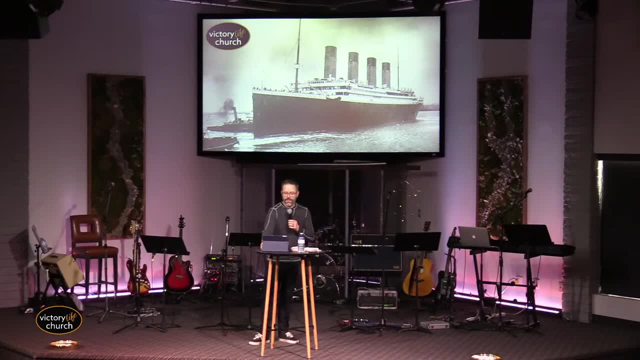 Man had conquered nature And that overconfidence that they had- man had conquered nature- Explains the electrifying impact that its sinking had upon the public and the world. Amen. There was even widespread disbelief when there was first reports of something happening. 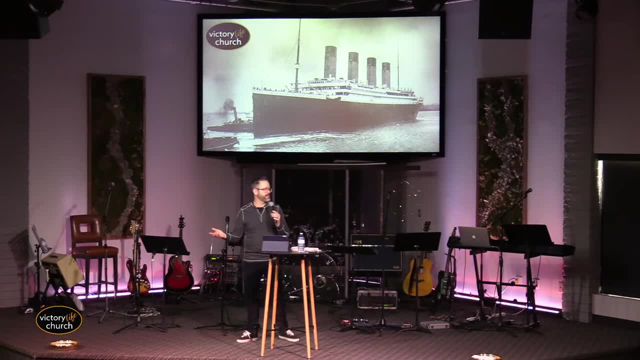 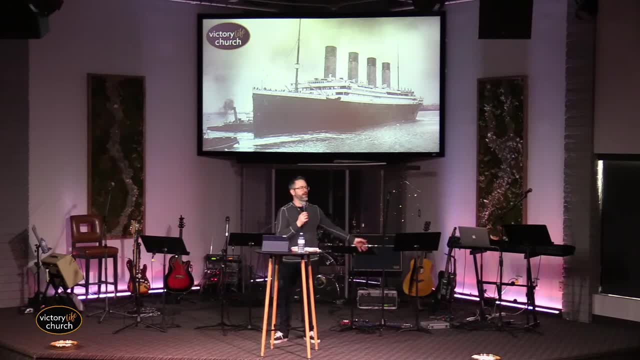 back in that day and age, misinformation abounded. Newspapers were reported. Newspapers were reporting that the ship had collided with an iceberg, but it was fine. They were just towing it back to port with everybody on board, And it took hours for accurate information. 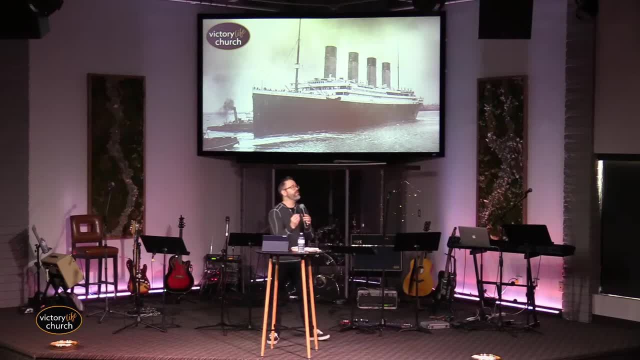 to actually even begin to become available. But even when they got that information, all these people had trouble believing and accepting that this paradigm of modern technology could actually sink. How could it actually sink? and not only sink but take 1,500 lives with her? 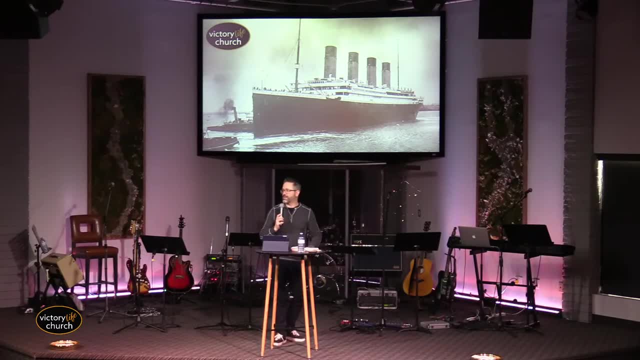 One ship historian compared the Titanic story because sometimes we can't really fathom that Now. most of us here were probably alive in 1986. Most of us And we were around for the Challenger disaster- and this historian compared it to the challenger space shuttle disaster and the world reeled at. 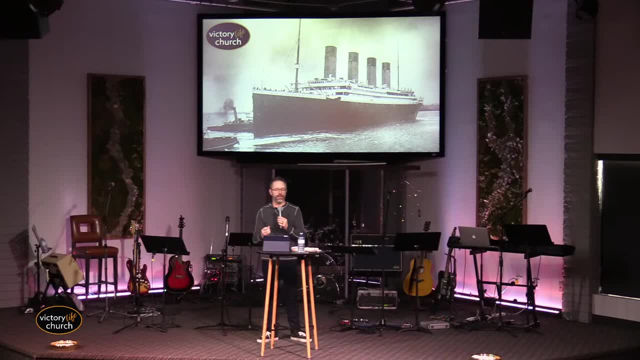 the notion that some of the most sophisticated technology on the planet ever created could actually explode into oblivion- oblivion before our eyes on national tv- and take all of its crew. and both of those tragedies triggered a sudden and complete collapse in confidence, revealing that we are vulnerable despite our modern presumptions of technological infallibility. 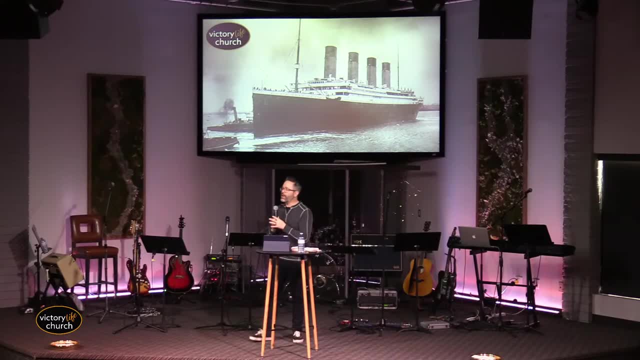 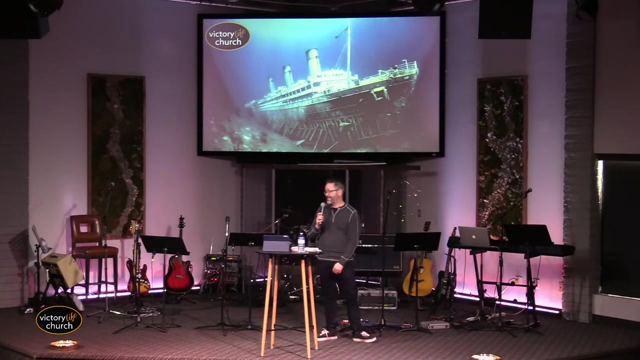 amen. and as we look closer, as you look closer at the titanic, there were many warning signs that could have prevented its sinking or could have at least saved thousands of lives had they been listened to. here's a couple of the warning signs. let's throw up that next picture of the titanic, because this is what it looked like. 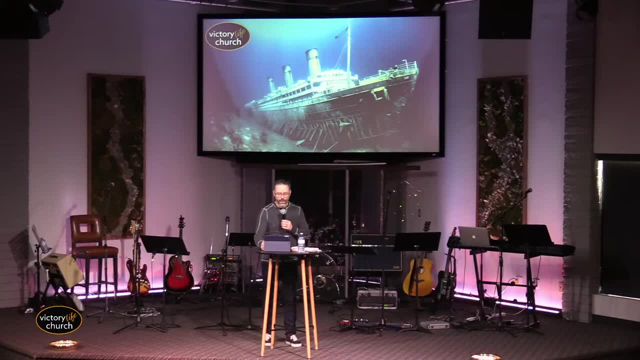 one of those warning signs was this: the olympic class ships. this ship featured a double bottom, 15 watertight bulkheads equipped with electric water gauge doors, which were could be operated right from the helm, one at a time or all together. they could close off if there was a breach. 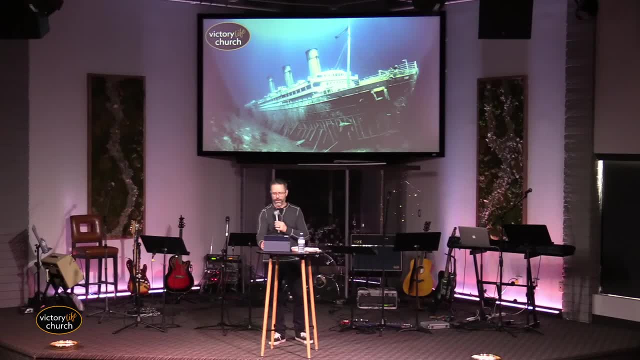 somewhere they could close it off. boom, boom, no problem, and they were inspired in shipbuilder magazine. but they realized that there was a design flaw and it probably was. a critical factor into the titanic sinking was, in fact, that at certain angles the water could flow over top of them. 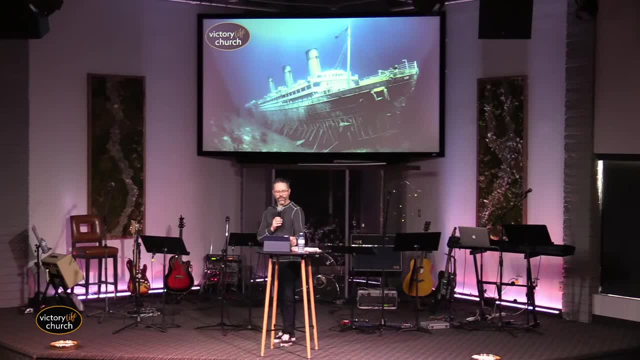 and, in fact, several of the titanic um the cunard company that owned the titanic one. some of their companies had already talked about innovative safety features devised to avoid that situation. now, had white star taken a cue from them, it might have saved the titanic. 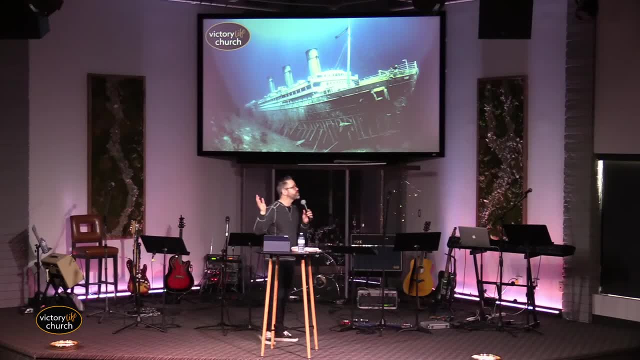 but they had already. they had already said no, this ship is unsinkable and you can't change our mind about it. second thing: one of the titanic companies that owned the titanic, one of the titanic companies, did what they thought about the air traffic니까. 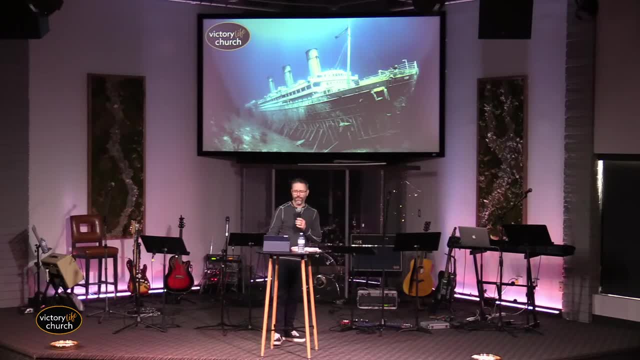 was the fact that, because it was the safest ship ever built, we don't need more than 20 lifeboats, only enough for 2200 passengers and crew, or for half of that 2200 people. this discrepancy rested on the belief that, since the ship's construction made her, 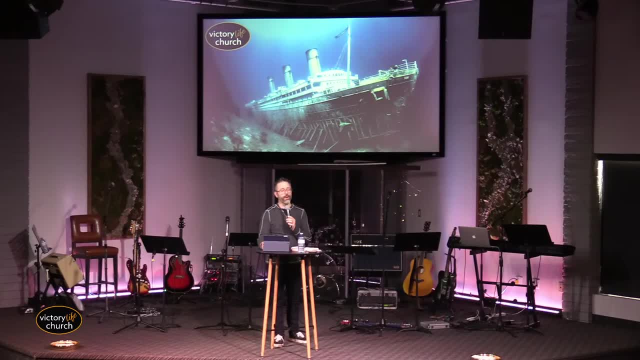 unsinkable lifeboats were necessary only to rescue survivors from other sinking ships. And you know what Lifeboats take: up valuable deck space. They canceled that very morning. They canceled the lifeboat drill scheduled to take place that very morning, April 14th. Hmm, You know what? I didn't even notice. 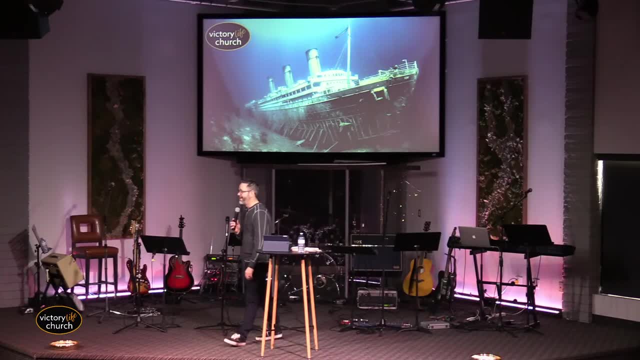 that that today is April 14th. That is not planned. Wow, April 14th 1912.. They scheduled a lifeboat drill, a drill to say hey in the event of a problem. this is our plan. 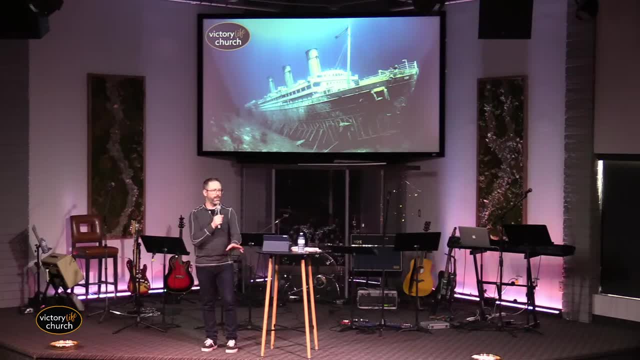 How many times do we go into our lives going? I don't need a backup plan, I don't need a safety plan, because this is an unsinkable idea. And then we use that phrase. Hmm, Seemed like a good idea at the time. 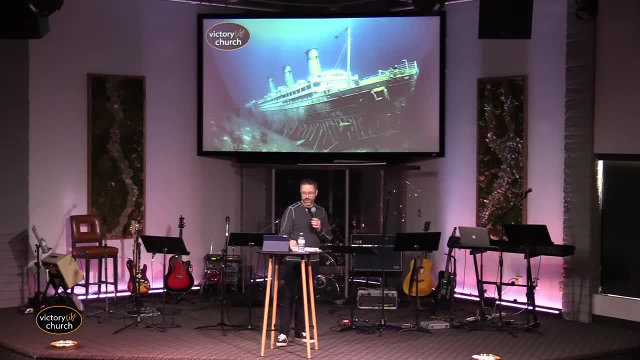 They canceled it. Maybe they could save more lives. Not only were there not enough lifeboats to save everybody, most of the lifeboats left the Titanic not filled to capacity. For instance, the first lifeboat to launch, lifeboat number seven, only carried 24 people. 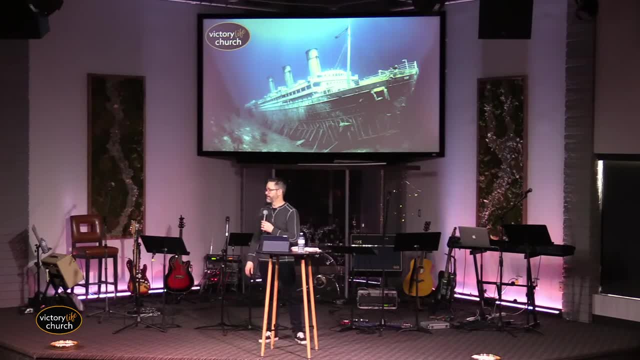 despite having a capacity of 65.. Two additional people later transferred the seven from five when they were out on the water Life boat. number one carried the fewest people, only seven crew and five passengers, So 12 people despite having a capacity of 40.. 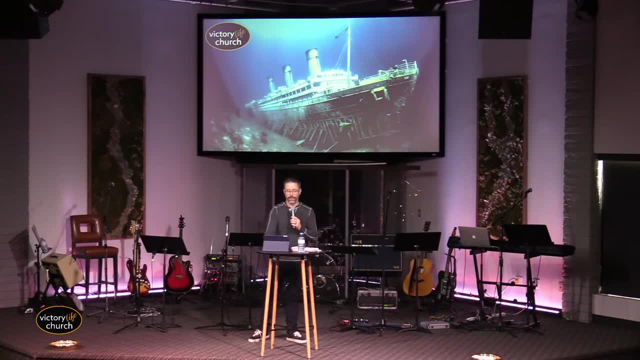 Another thing: there was another boat, closer than the carpathia, to rescue them, the californian. yet they didn't respond until it was much too late, because they saw mysterious lights in the sky from the flares being set off by the titanic, woke up their captain to tell him, but he didn't issue any orders because, yeah, you know what? 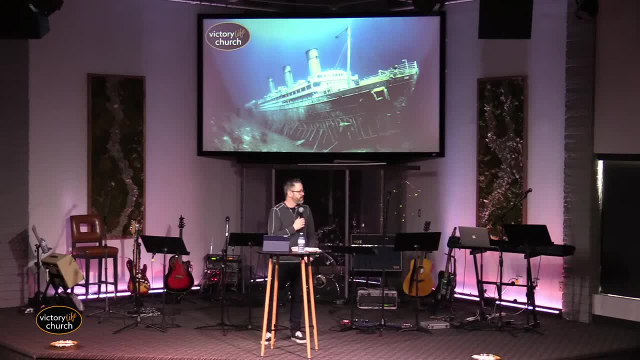 the ship's wireless operator. he's already gone to bed. we don't want to wake him up. and then they didn't know about the distress signals to the next morning, but by then the carpathia had already picked up whoever remained, and probably one of the most significant warnings. 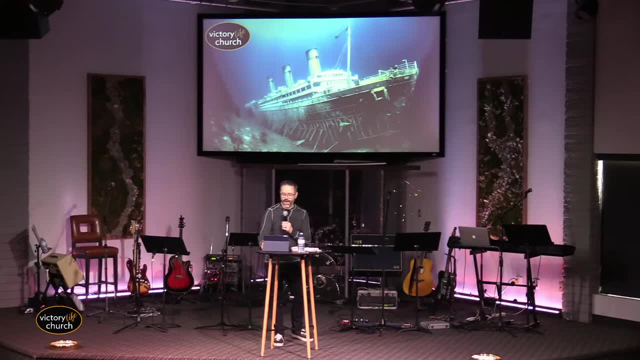 throughout the day on april 14th, the titanic received a number of wireless messages from other ships warning about icebergs along their path. is that ringing and turning on a light bulb for anybody right now about messages we get about icebergs in our path and we go? 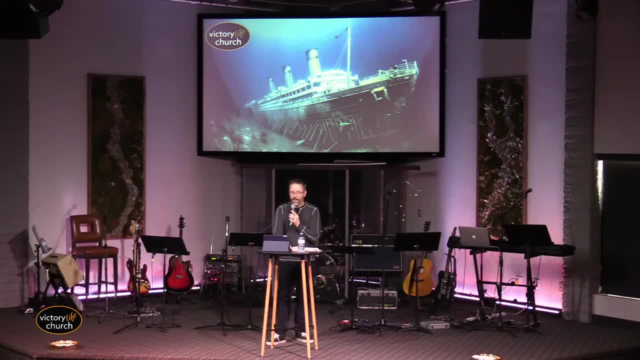 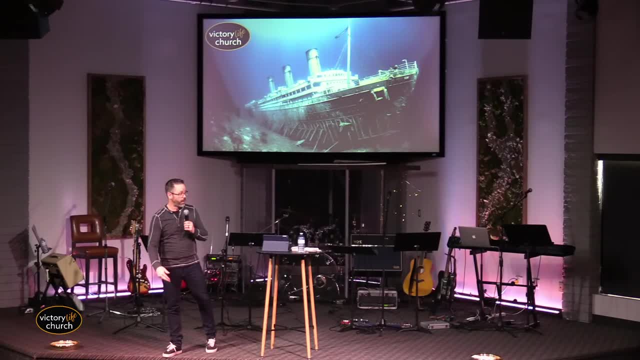 foot, stepping on a mouse trap and not getting to your breath, saying there might be some more after that. now the captain, unaware of how serious the warnings had become, went to bed at 9: 20 the lookouts had been told. well, you know, be a little bit more diligent in your observation. 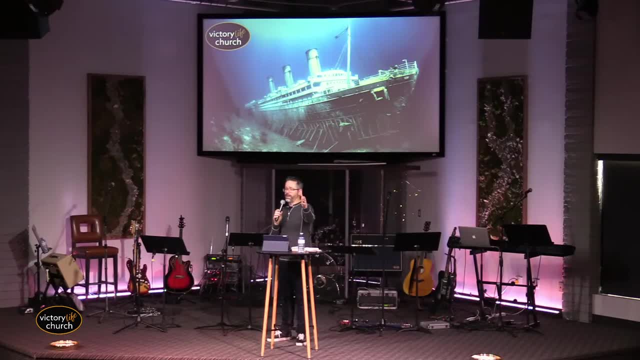 but they were still steaming full speed ahead, hitting the iceberg. now, that night was cold and clear, but the moon wasn't very bright. That coupled with the fact that the lookouts didn't have binoculars. So imagine being in the lookout and you're standing on the edge of a ship. 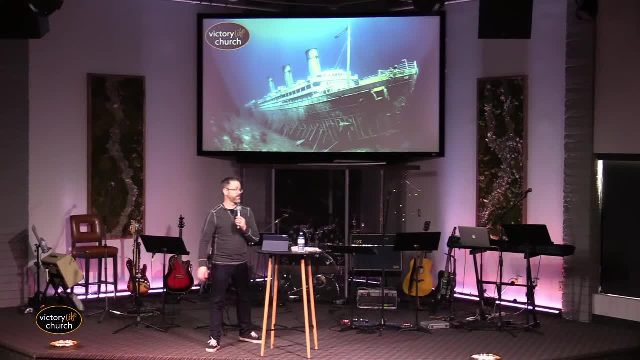 and you're supposed to watch for icebergs in the dark With no binoculars. you got just a subtle, So they only spotted the iceberg when it was directly in front of the Titanic. From the time that they spotted the iceberg, they had 37 seconds. 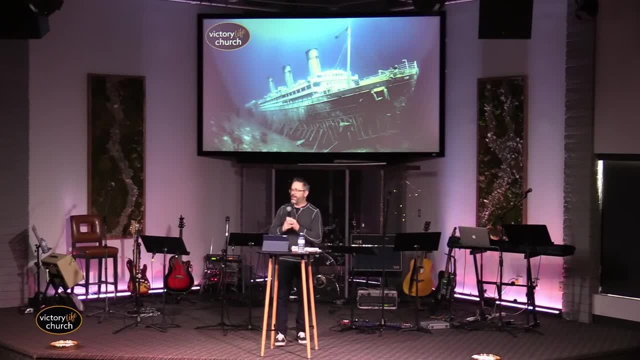 Until impact, They hadn't equipped themselves to see Man. this is good. How many times do we not equip ourselves to see what is in front of us? God has given us binoculars to tell us: if you go this way, this is what will happen. 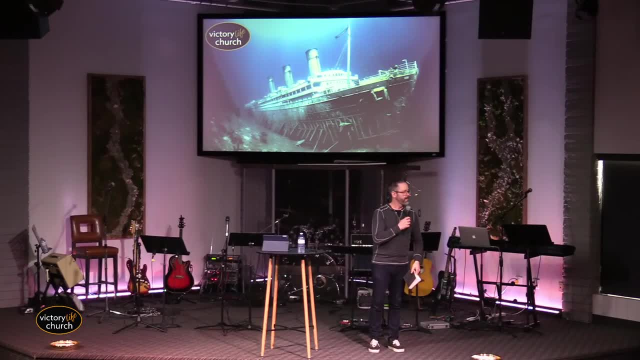 If you go this way, this is what will happen And we're like, oh, I'm going to go this way anyway, Because we don't put on the binoculars, We don't equip ourselves, We don't equip ourselves to see what needs to be seen in front of us. 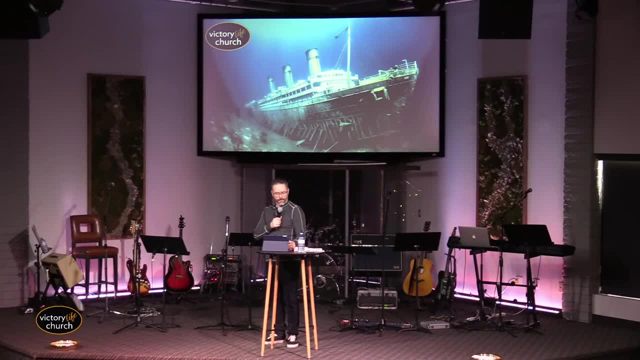 Hallelujah. Thank you, Holy Spirit. All these warnings, yet man's understanding or desired purpose caused them to ignore them. Their desire to get that unsinkable ship across the ocean caused them to not look and see, And you could call it pride. 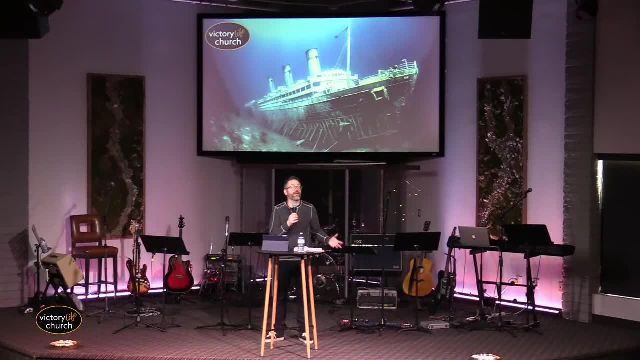 You could call it arrogance, In some instances maybe even ignorance, not understanding. But they didn't heed the warnings And many storms or problems in our lives could be lessened or avoided altogether if we follow the leading of the Holy Spirit, That still small voice inside that goes. 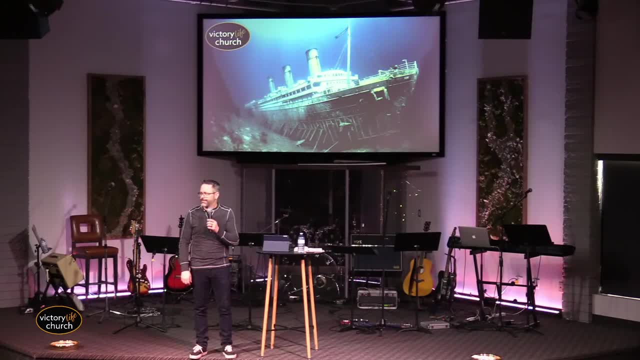 this is a good idea. And that voice goes: hmm, Hmm. So many times we're waiting for God to jump out with a giant stop sign and go- hey, Don't be dumb. But instead he's going. hey, probably not such a good idea. 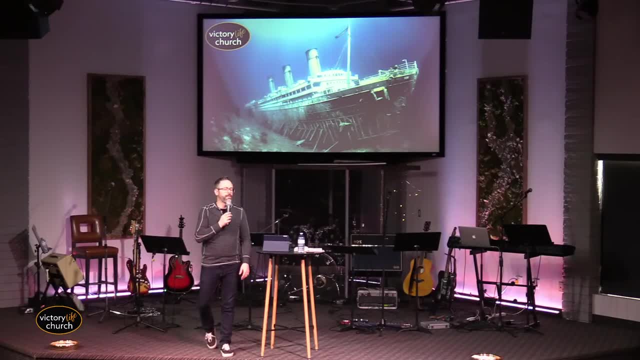 But hey, you have free. will I love you enough to give you free? will I love you enough to allow you to make your own decisions? I love you enough to allow you to choose me. I'm not going to make you choose me. 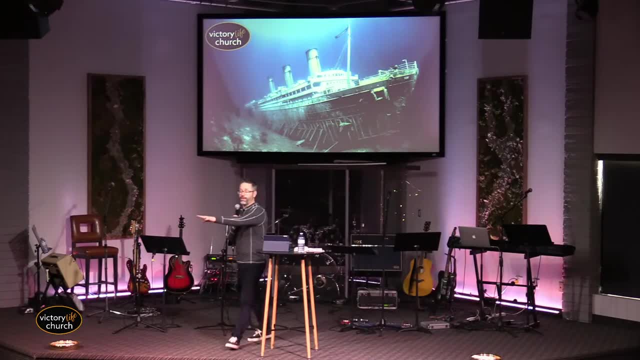 I'm not going to make you choose the right path. I'm going to show you, I'm going to be the light unto your path. I'm going to give you the path that leads to life. I'm going to do all these things, but I'm not going to make you do it. 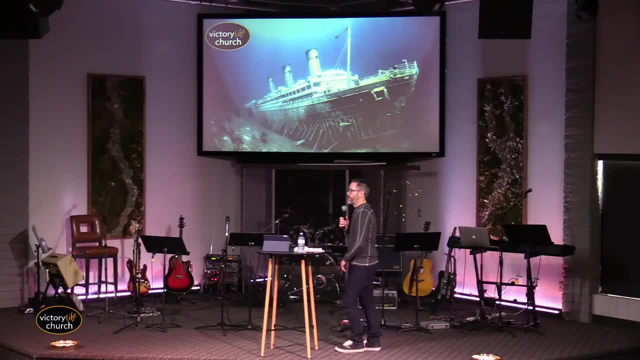 I'll be right here by your side to walk with you. Daily, we're faced with decisions, small and large, that have lasting effects upon our lives. Don't we? Some things that we think are the smallest decisions, yet have the biggest impacts on the future? 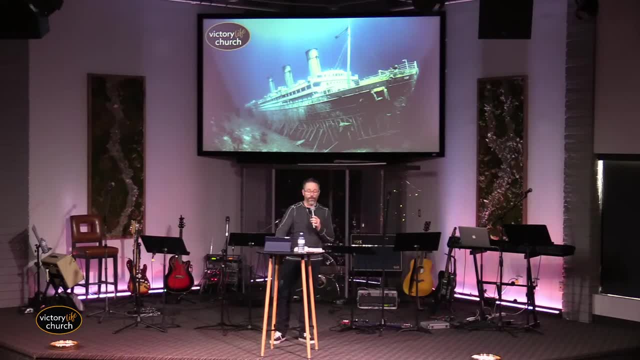 Man, there's probably, There's probably a good chance that you are going to, or already have made some choices that have not resulted how you thought they would. But be encouraged Why? Because Holy Spirit will never leave you nor forsake you. 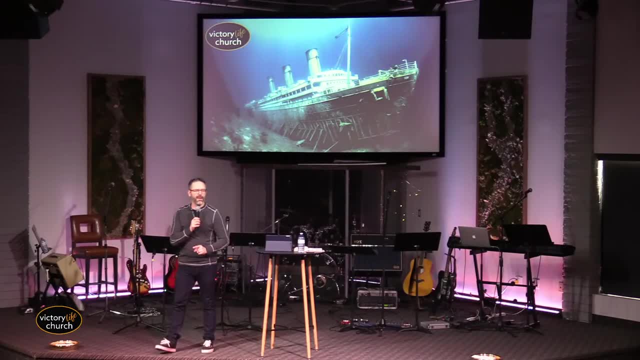 Amen, He walks with you. When you come to that option and there's door A and there's door B and God's plan is door A and you're like that's pretty And door, But door B looks So good And you walk through door B. 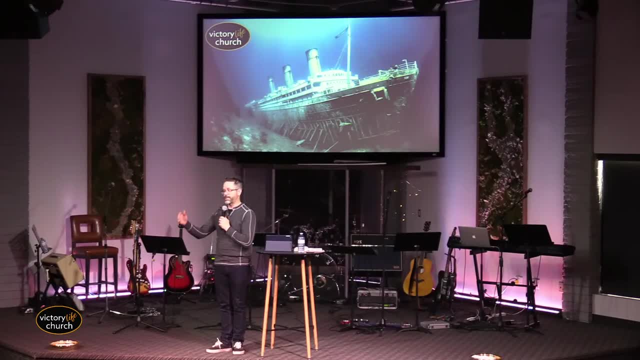 Holy Spirit's like not going. oh man, see ya. No, he says okay, I'm coming with ya. And you get to the other side and you're like: oh, look, how great the grass is over here. Oh, my goodness, it's because they fertilize it lots. 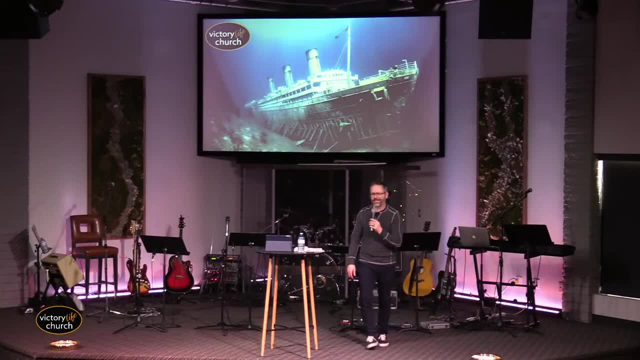 and there's all sorts of poop over here and I don't like it and it's sticky and smelly and gooey and oh ah. And Holy Spirit's like: hey, I'm right here, Here's another door, Here's another door. 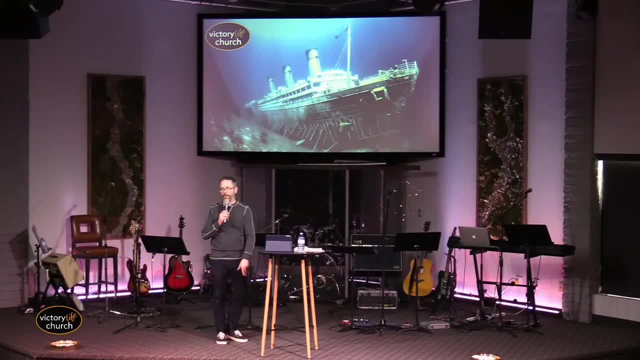 Which one would you like to go through? Here's the one I think you should go through, But you choose. And he never leaves us nor forsakes us. He's always there to lead us back on track. Amen, If we're the captain of our own ship. 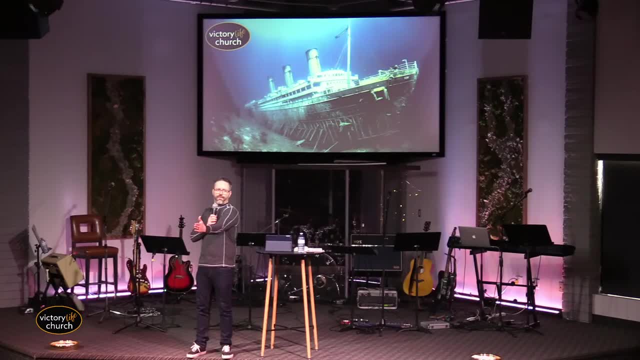 and we set our course one degree off doesn't feel like very much, does it? And if you turn your car one degree, you're okay. But if you set sail from New York towards England and your compass is one degree off, 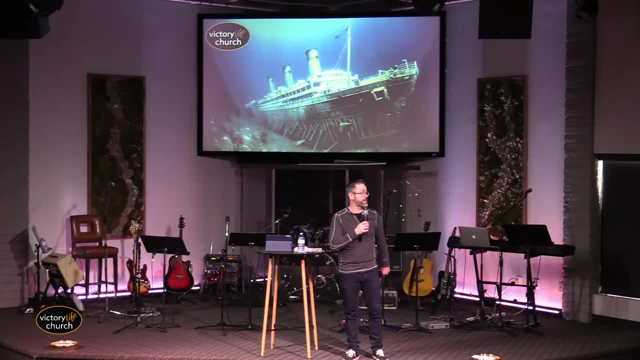 you're going to be a long ways from England by the time you get across the ocean, Amen. And sometimes we find ourselves we're making those one degree mistakes, We're making those one degree judgments for our lives, And then we're like God: how did I get here? 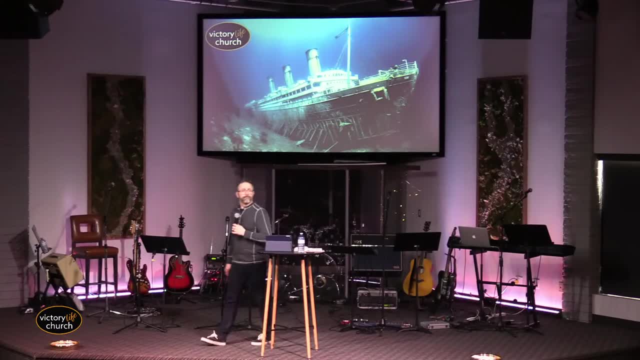 Where am I? This is not London, This is Afghanistan. How did I get here? One degree, That's all it takes is one degree for a long period of time, But Holy Spirit's always there. You know what? I'm right here. 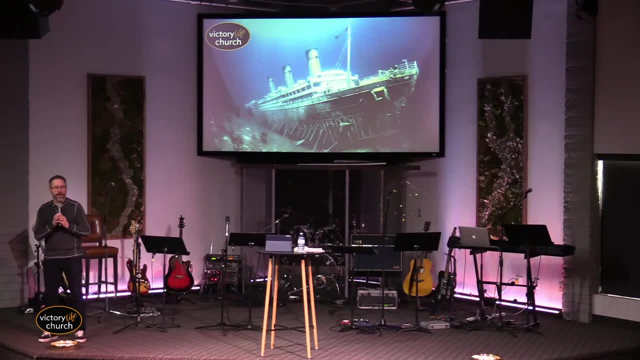 And we get way over here. We're supposed to be there. We get way over here And we're like, oh, I got to do this, And we throw the steering wheel right. I'm going to fix it all right now in my life. 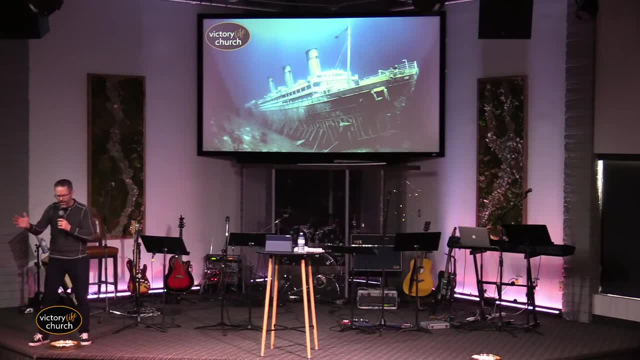 Anybody ever done that. These are all the things I've been doing wrong, And it's like I'm just going to fix it all now And the boat tips over and you're in the sea And you're even worse off than you were before. 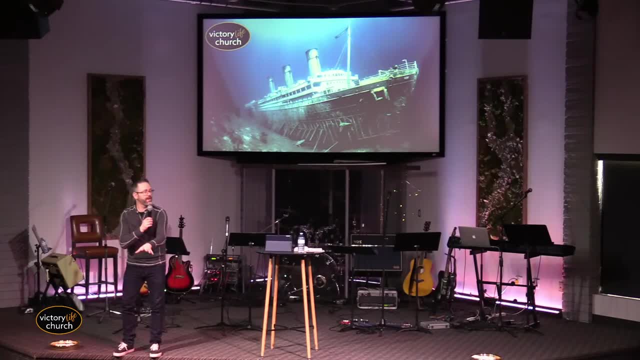 Wow, this is all free, because this is not my message. But Holy Spirit is there to go. you know what? Let's just start one degree at a time. That's the love of God. He says you don't have to fix it all right now. 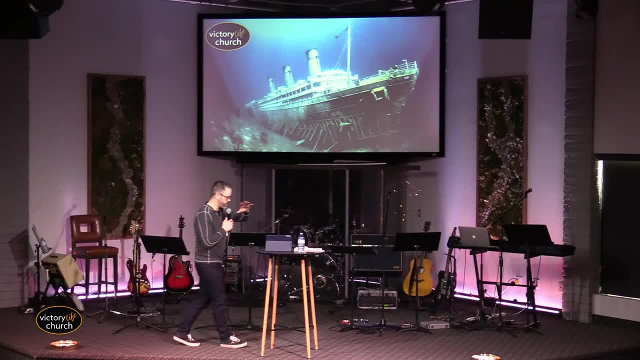 Trust me, Begin to get to know me. If you're walking through life, you're watching online. you're walking through life right now and you don't know Jesus as your Lord and Savior and you're over here going. I should be over there. 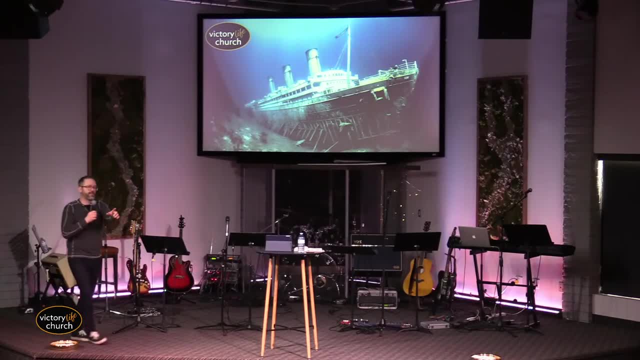 Why am I not there? And you've got all these things in your life. Holy Spirit says: just come, get to know me God. God says: just start by asking Jesus to be Lord. Come, get to know me one degree. 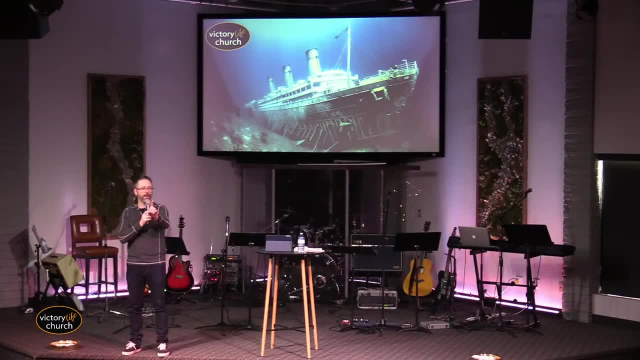 Don't worry about all the things that have led you off path one degree. Give me your heart and I'll begin to lead you back, And we'll sail your ship right back to where you're supposed to be. amen, Amen, That's who Holy Spirit is. if we'll listen. 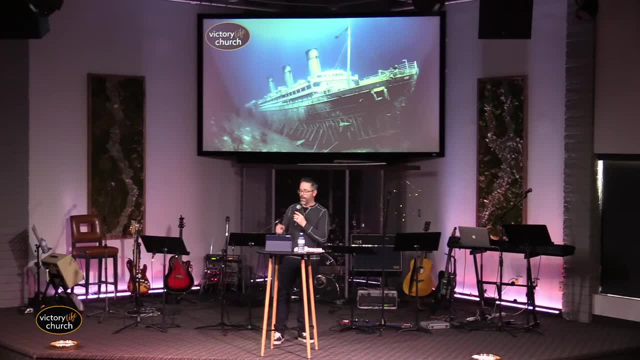 The Titanic was a result of poor decisions and the loss of life was great. But today I want to look at another shipwreck in the book of Acts, Acts 27.. I don't have all the scriptures for you today because we're going to look at Acts 27, verses 7 to 44.. 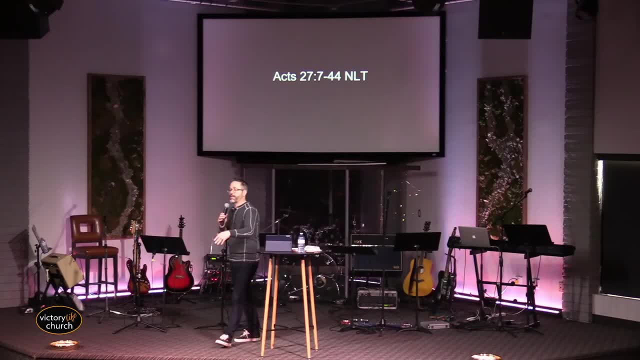 I will read them for you, but I want you to go home. I want you to look at this. I want you to see re-listen to this message. make notes, find out what you're looking. Acts 27, verses 7 to 44.. 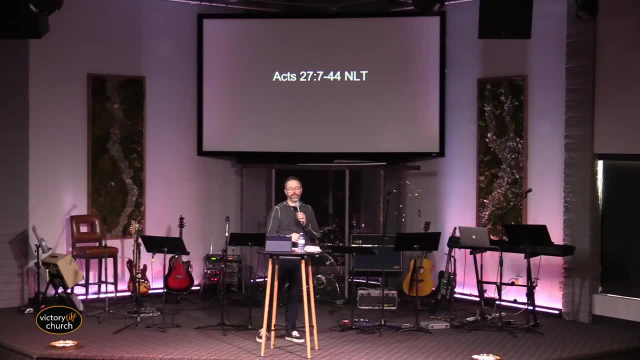 Here we have the Apostle Paul. He's a prisoner on a ship bound for Italy. So Paul is a prisoner, So he's not the first person you would expect anybody on that boat to listen to for direction, right? Amen, Realistically. 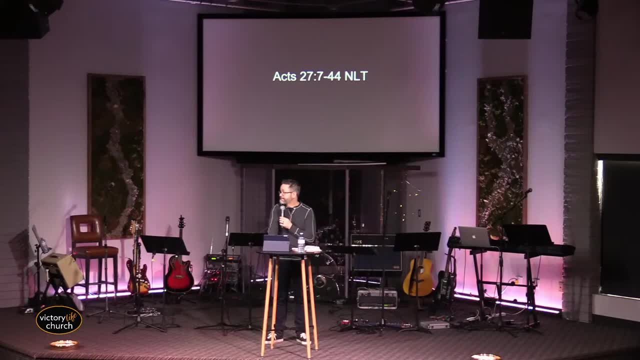 that's the Holy Spirit in most people's lives: A small yet powerful voice, if we will listen. So let's look at this. Acts 27,, starting verse 7,, says this: That sounds like what's going on in my sinuses right now. 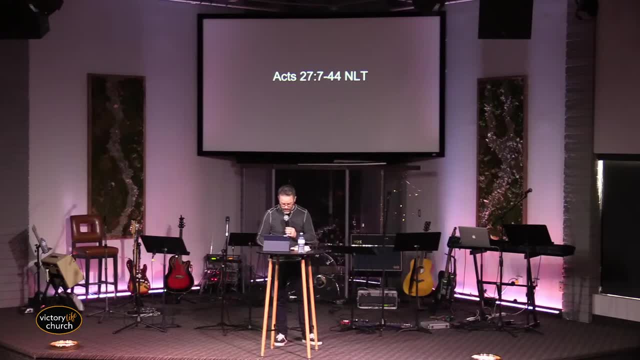 But the wind was against us. so we sailed across to Crete and along the sheltered coast of the island past the Cape of Salmon. We struggled along the coast with great difficulty and finally arrived at Fairhavens near the town of Lycia. 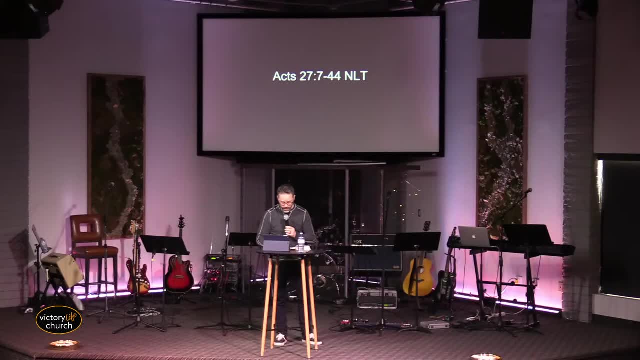 We had lost a lot of time. The weather was becoming more and more bad. It was becoming dangerous for sea travel because it was so late in the fall And Paul spoke to the ship's officers about it. So here's, Paul a prisoner. 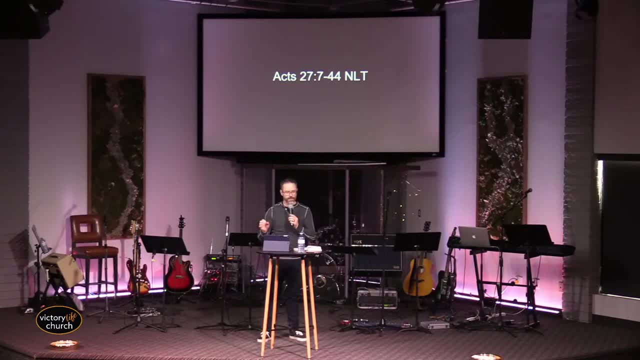 He's kind of like the Holy Spirit right in the moment. He's the Holy Spirit speaking into lives. We're at a place where decisions need to be made. This ship is at a place. they got to make a decision right now. What are we going to do? 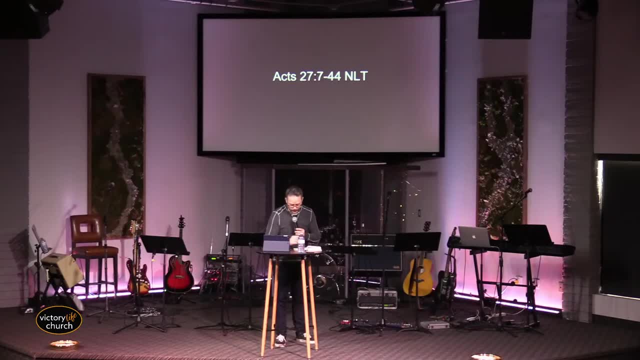 And so Paul says this in verse 10. He says: I believe there is trouble ahead if we go on. There should be bells and whistles and sirens going off by that time, right Shipwreck, loss of cargo. 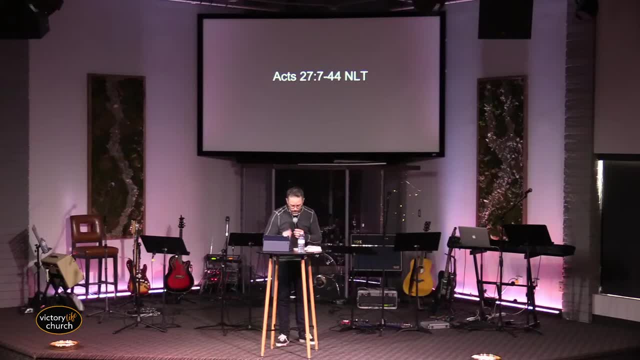 and danger to our lives as well. But the officer in charge of the prisoners listened more to the ship's captain and to the owner than to Paul, And since Fairhavens was an exposed harbor, a poor place to spend the winter, most of the crew wanted to go on to Phoenix. 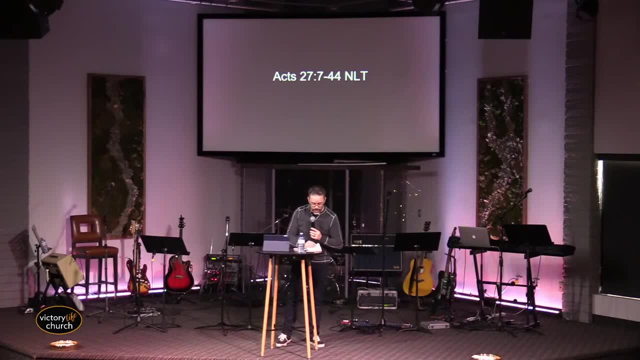 farther up the coast of Crete And spend the winter there. Phoenix was a good harbor with only a southwest and northwest exposure. Now we note the ship's captain is the one guiding the ship right. That's us. We are the captains of our own ships. 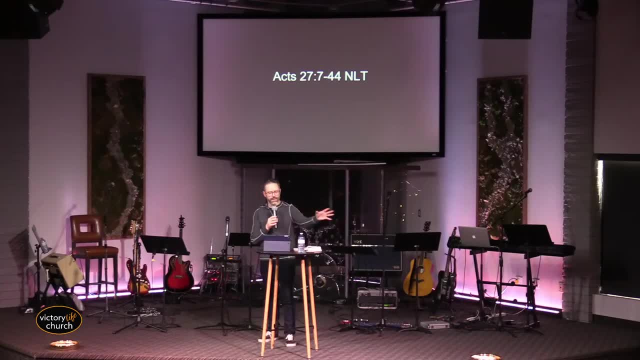 God has given us the authority to be the captain of our own ship And we look at the situation around us. We look at what we think is best And we generally don't base our decisions on what God says. But we see and we feel right. 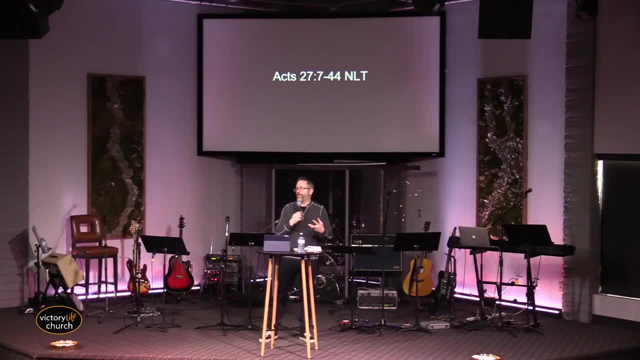 We see things, we feel things And it looks good. Therefore it must be good. Well, the design of the bulkheads on the Titanic looked good, seemed good. A quick side note: Hebrews 5.14 says that solid food 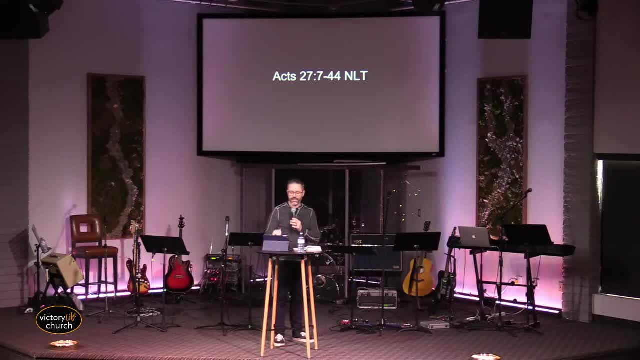 is for those who are mature, who, through training, have the skill to recognize the difference between right and wrong, Good and evil. If good is so easy to see and so easy to discern, then why does it take training and skill to recognize the difference, according to God's word? 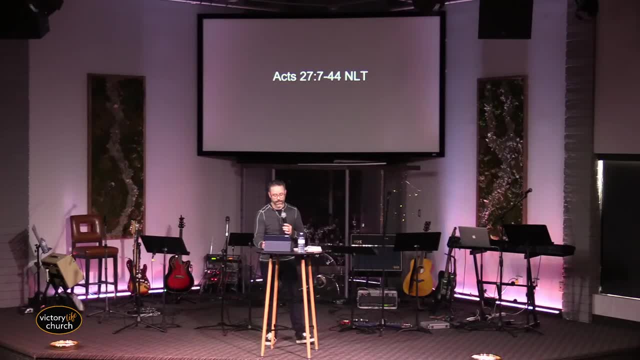 Amen. There's something in that, When we set sail in our lives toward a destination that looks favorable, despite the Holy Spirit warning us not to, we end up in a storm. And I read this, I read this quote from John Bevere one time: 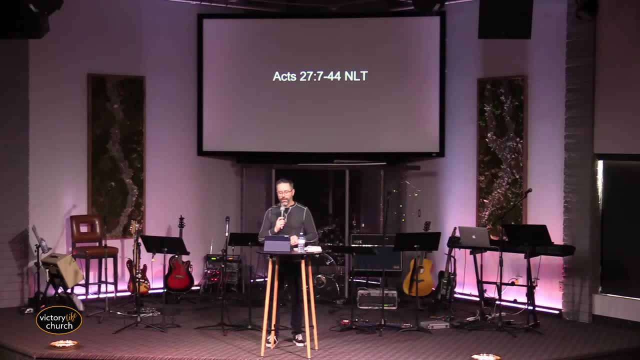 and it was powerful. Anything outside the will of God is not good. No matter how good it looks, it will always lead you somewhere you do not want to be. No matter how good it looks, it will always lead you somewhere you do not want to be. 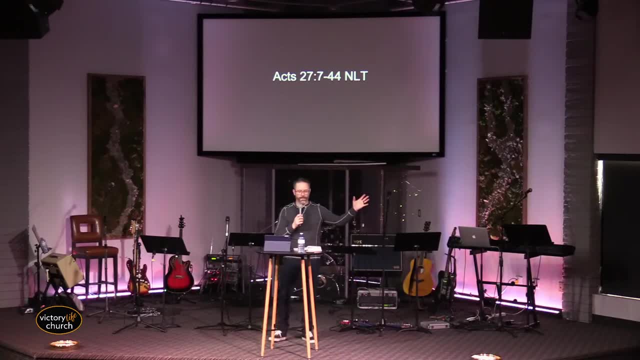 We probably all have an experience with that, Amen. If you're not old enough to have that experience yet, you're not old enough to have that experience yet- Follow the Holy Spirit, so you don't have to. So I want it into verse 14.. 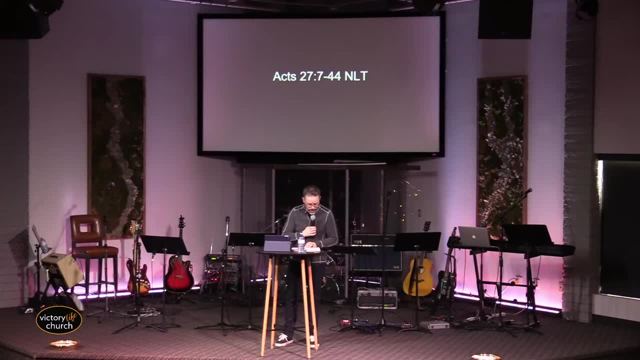 Where am I here? Flip the page. Well, in verse 13 it says: when a light wind began blowing from the south, the sailors thought they could make it, So they pulled up anchor and sailed close to the shore of Crete. 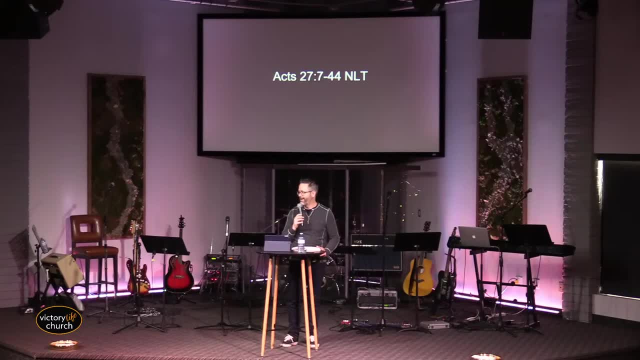 But the weather changed abruptly. My goodness, Anybody else here have some sort of story in their life that they're thinking about, That they're thinking of right now. I'm like, oh yeah, we thought, oh, I can make it. 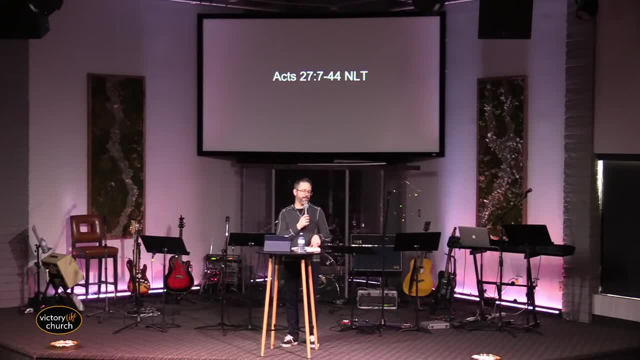 I've had gas stories of that. Oh yeah, we can make it That many kilometers to empty Ring ring. Hi, Corey, I'm out on Highway 16 and I'm out of gas. Can you bring me a jerry can? 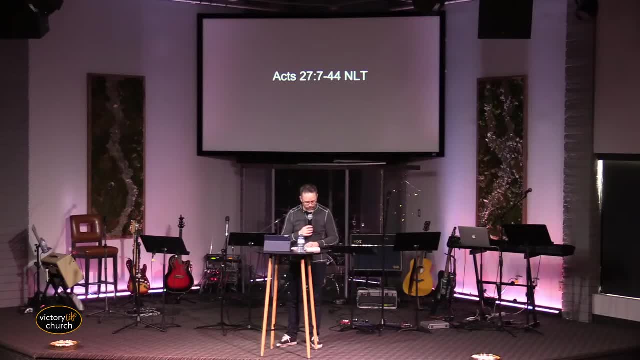 But the weather changed abruptly and a wind of typhoon strength called a northeasterner burst across the island And blew us out to sea. All of a sudden, you find yourself in a situation in which the conditions are declining rapidly and we struggle to try and gain control. 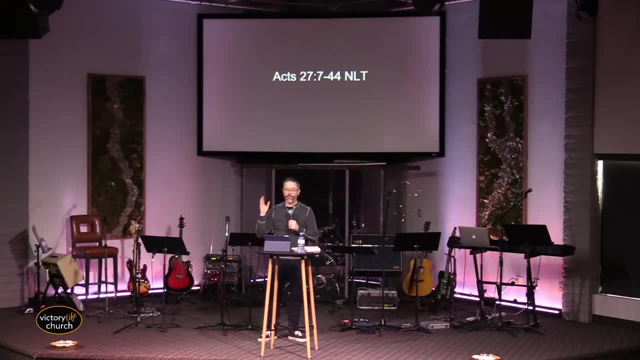 I'll tell you what things are happening all around us today: that if we're not grounded and led by the Holy Spirit, we're going to end up in fear, struggling to find a firm foundation to stand on. We're going to be out in sea. 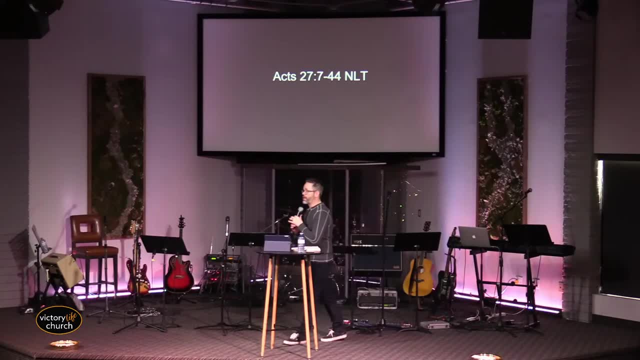 looking around and all we see is water and nothing solid to stand on. if we're focusing on what's going on And around us today, you focus on what's just happening again in Israel right now, Iran launching attacks. Man, if you start looking at that stuff, 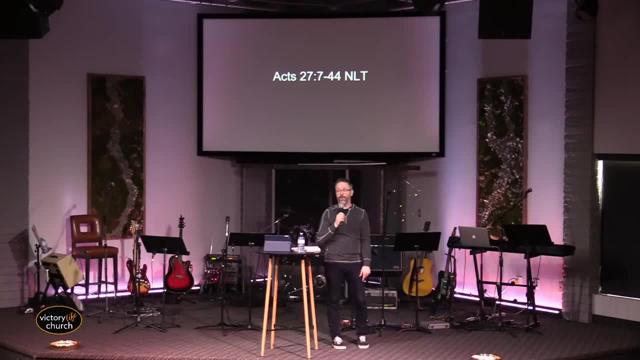 without being grounded in the Word and being led by the Holy Spirit, you'll be like: oh, what is going on? Verse 15 goes on to say this: the sailors couldn't turn the ship into the wind, so they gave up and let it run before the gale. 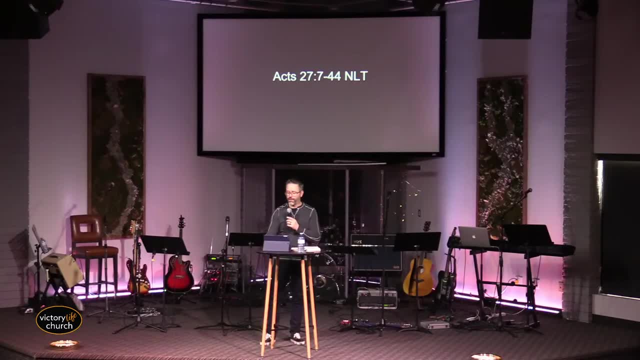 So many people find themselves, when they're functioning in their own strength, unable to turn the ship into the wind. See, when you turn a ship into the wind, you turn it against. That's what's pushing you away further, And so they give up. 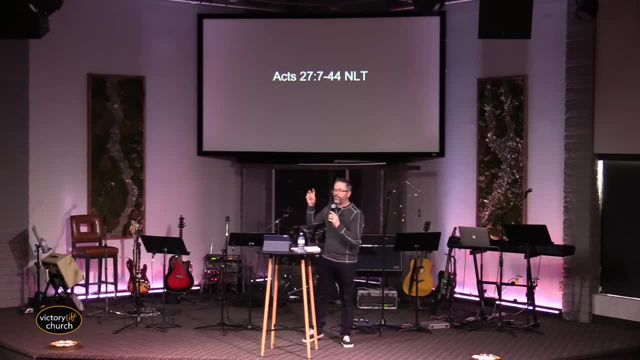 and we let our ships run before the gale, And what that means is we let our lives be pushed wherever the storm or the circumstances send us. And that's what these guys did. They're like: we can't do this. We can't do this. 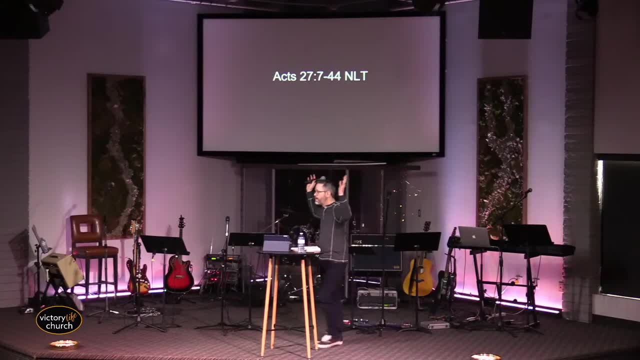 We can't get this straight. We can't whatever Verse 16 says. we sailed along the sheltered side of a small island named Kauda where, with great difficulty, we hoisted aboard the lifeboat being towed behind us. Then the sailors bound ropes. around the hull of the ship to strengthen it. They were afraid of being driven across to the sandbars of Syrtis off the African coast, So they lowered the sea anchor to try and slow the ship and were driven by the ship. They were driven by the ship. 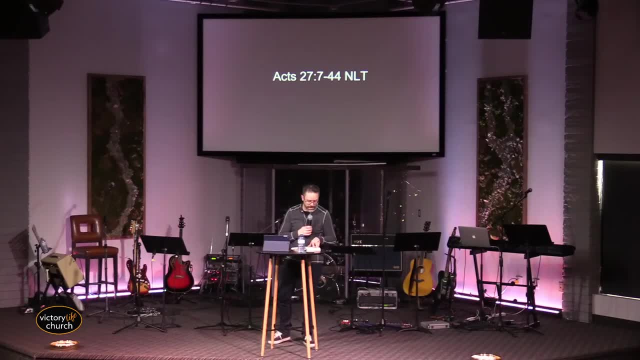 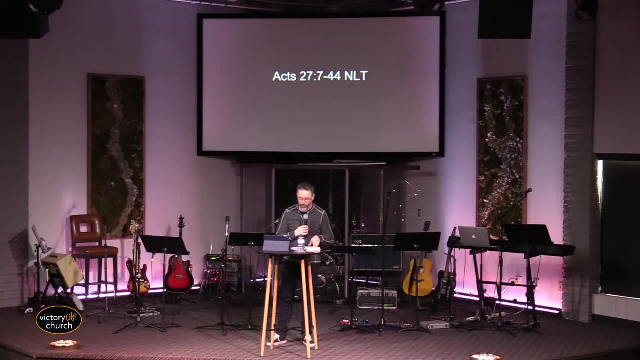 The following day they even took some of the ship's gear and threw it overboard. See here in verse 16 it says we sailed along the sheltered side and they pulled in the lifeboat. And we get to a place when it seems like 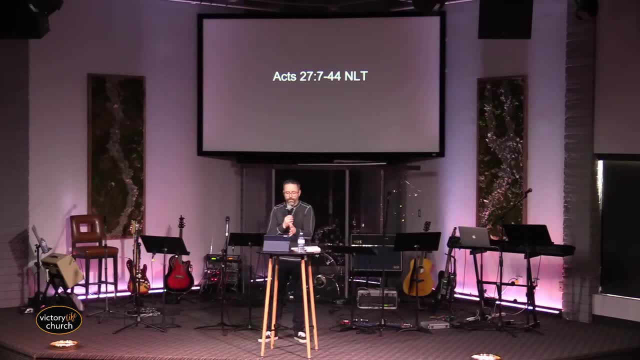 we have a little bit of a break in the storm right And we pull close that which we think will help save us. They pulled in their lifeboat. You know it's difficult, but we pull those things close If your storm is financial. 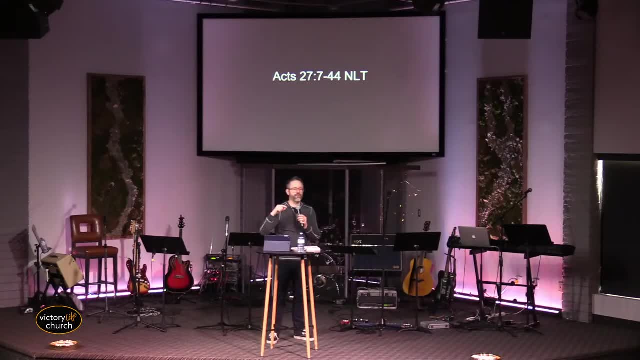 maybe because of a poor decision. the first thing we generally do, without talking to God, is to tighten up the finances. Stop giving, drop our responsibilities and commitment in order to take extra work on. so we can make more money, We try to tighten the strings around our ship. 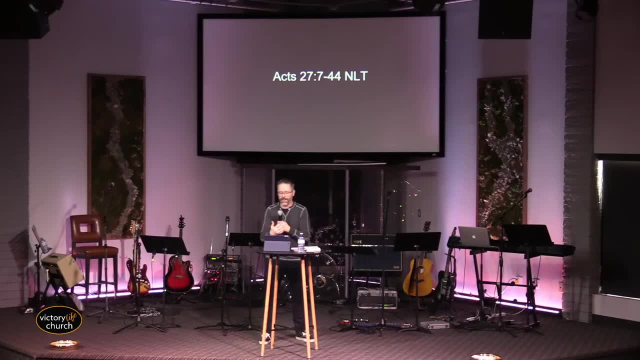 They wrapped ropes around the front of the ship to try and tighten it for stability. Now, if God's telling you tighten up the ship strings, that's what you do. But that should be because God is telling to you. But we need to be sure it's God. 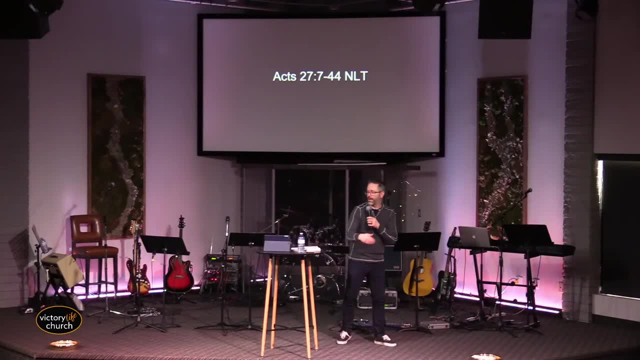 because otherwise we get caught deeper and deeper and deeper. And as things continue- in verse 18 and 19- and the storm rises, rises up again, they begin to throw things overboard, and we begin to throw overboard important things trying to stabilize our boat. 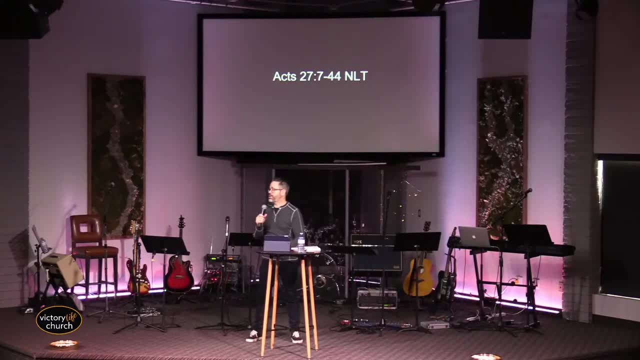 They're throwing the cargo and the ship's gear. For us, the ship's gear and the cargo could be family time, Things that we're like you know what? I can make that up tomorrow. Sometimes you don't get it tomorrow. 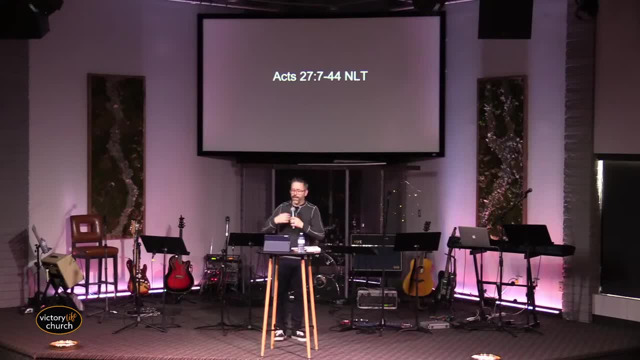 We begin to do everything we can think of in our own strength to lighten the load and stabilize the ship, Until verse 20.. The terrible storm raged for many days, blotting out the sun and the stars. The last line says: 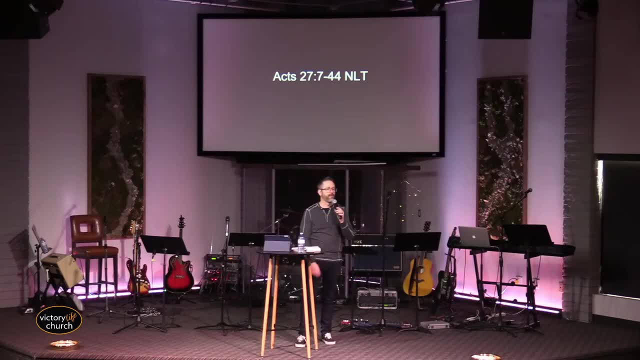 until, at last, all hope was gone. Until, at last, all hope is gone. Man, I don't know about you, but this sounds like a Titanic story, doesn't it? What a downer. And then verse 21 says: no one had eaten for a long time. 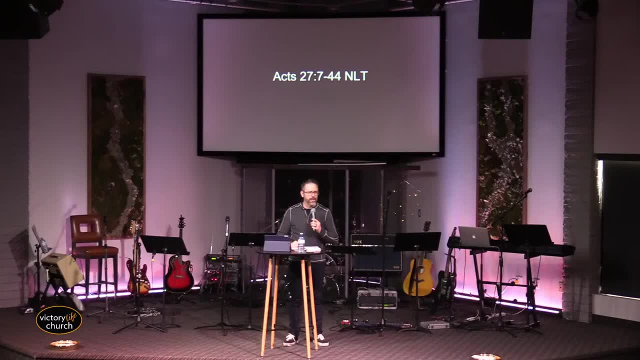 Finally, Paul called the crew together and said: men, you should have listened to me in the first place and not left Crete. You would have avoided all this damage and loss. Paul comes, and he comes with conviction. And at that moment, 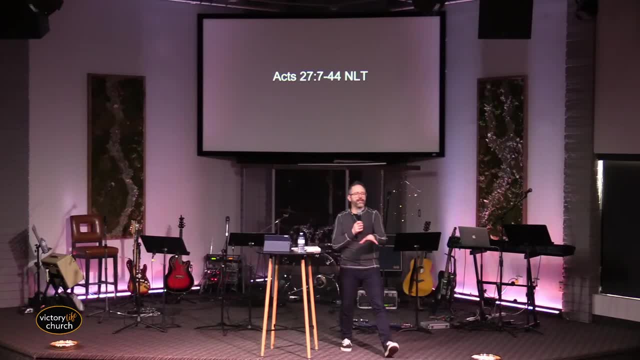 when we're in a place where all hope is gone and we're looking at a situation where we maybe have made a bad decision, we have an opportunity where Holy Spirit will come and speak to us and he might bring some conviction, and he might say: 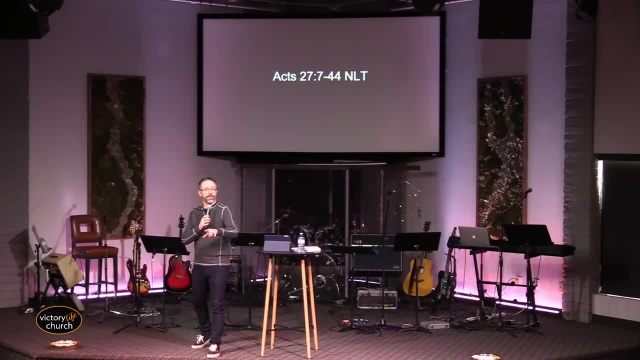 if you listen to me, you wouldn't be here. so listen to me now. And we have an opportunity, a choice here. We can have conviction or we can go to condemnation. Yes, pastor, I really messed up. I didn't follow the Spirit's leading. 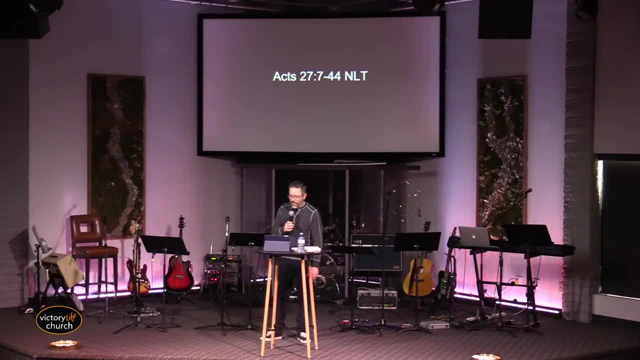 Now all hope is gone And I feel like I'm on the Titanic and all the lifeboats are gone. But I want to tell you this: Wait Before you allow conviction to turn to condemnation. keep going, Keep going, Keep moving. 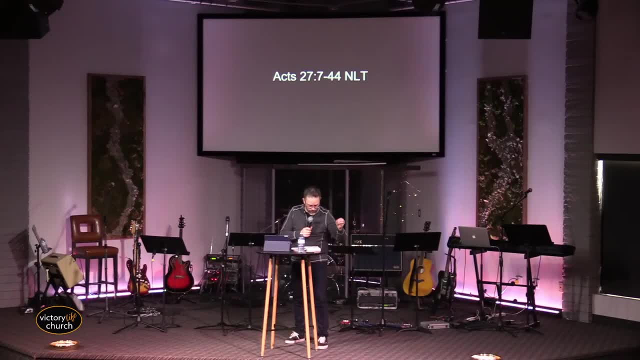 Keep listening, Because in verse 22, we lead up to it- It says: you would have avoided all this damage and loss. And if we stop there, we're like, yeah, I know, I could have. I'm such a loser. 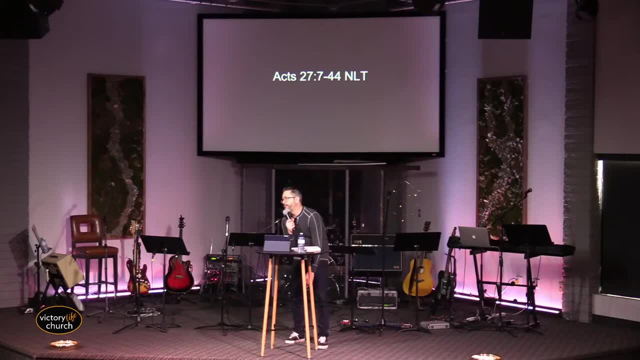 I'm not very smart. God, I'm dumb. Come on, You can't be the only one in this room that's ever thought they were dumb before, or somebody said that you were dumb. Well, guess what? That's a lie of the devil. 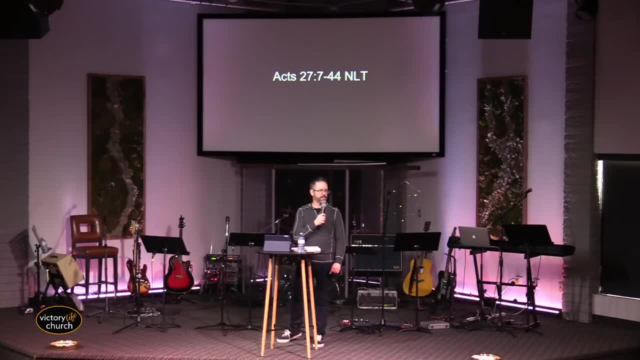 And when you speak it over yourself, you're lying just like the devil to yourself, Because verse 22, he says: but take courage, Take courage, None of you will lose your lives, even though the ship will go down. Well, that sounds encouraging. 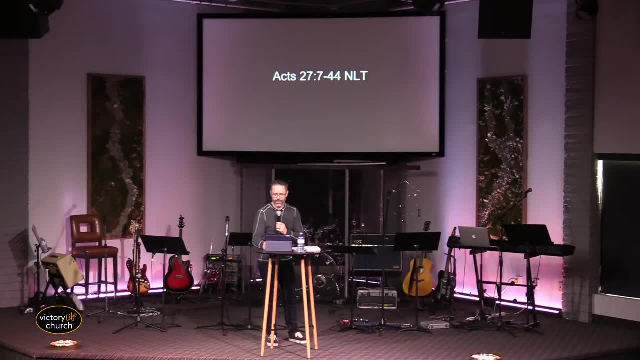 Wait what? Take courage. Remember the Holy Spirit is with you and will never leave you or forsake you. No matter which door you walk through, he's with you. He is with you, Amen, Amen And 1 Corinthians 10, 13,. 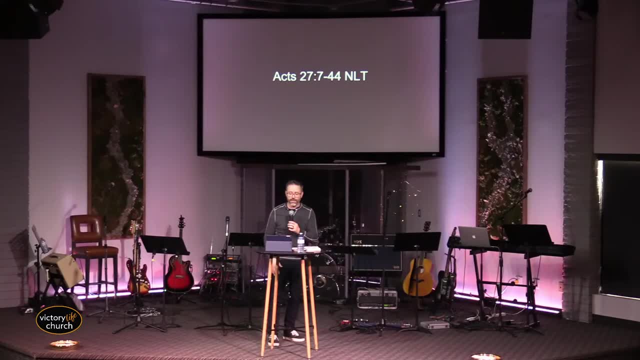 tells us in the Amplified Version- we looked at this a few weeks ago- for no temptation, no trial, regardless, as enticing to sin, no matter how it comes or where it leads, has overtaken you and laid hold on you. that is not common to man. 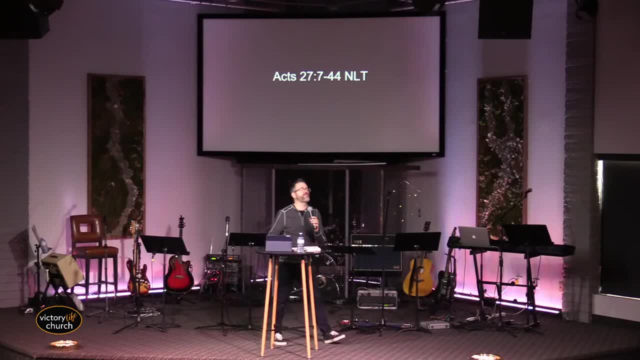 So it's not. you're not the first one, But God is faithful And he will not let you be tempted and tried and assayed beyond your ability and strength of resistance and power to endure. Why? Because the same spirit that rose Christ from the dead 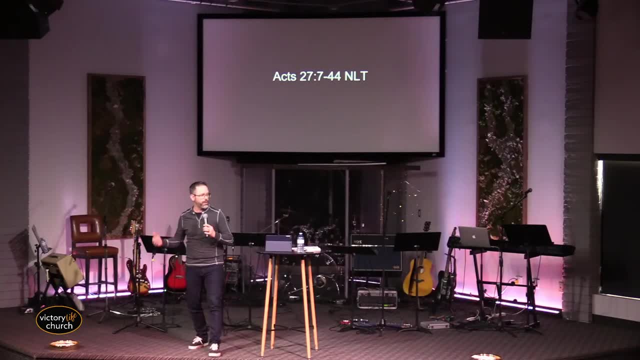 dwells within us and gives life to our mortal bodies. The joy of the Lord is our strength, Amen. Faith is hope of things not seen, And he will not let you be tempted and tried, But with the temptation he will also provide the way out. 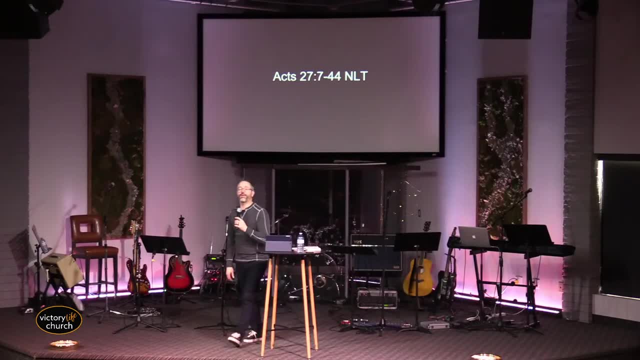 Hallelujah, Hallelujah, Hallelujah. There will be another set of options And you can choose again. And if you mess it up, you can choose again And again. And some of us again. The Israelites did it for many, many years. 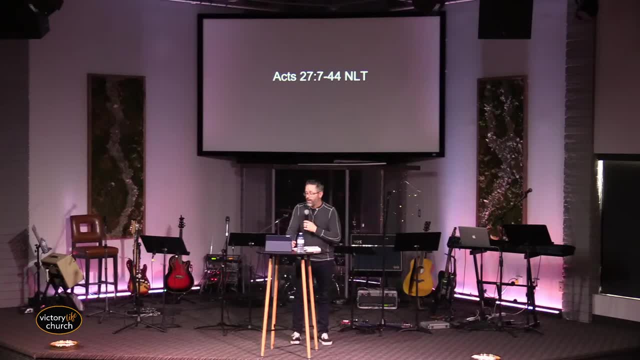 How come I'm not getting anywhere? Well, that made me dizzy. He says he will provide the way out, the means of escape to a landing place that you may be capable and strong and powerful to bear up under it patiently. Paul was still on the boat with them. 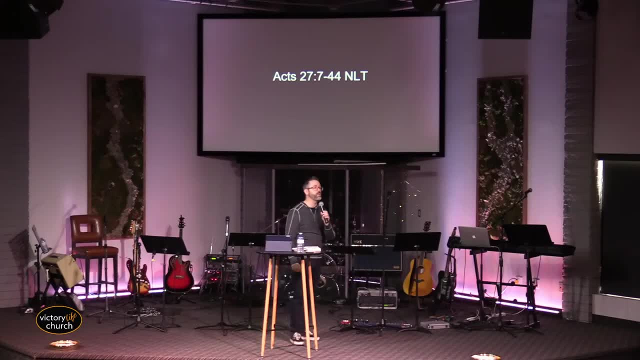 The Holy Spirit is still there and will lead you out of the mess if you listen to him Now. verse 25.. We'll keep going through 23.. It says: For the last night, an angel of God came and he said: Don't be afraid, Paul. 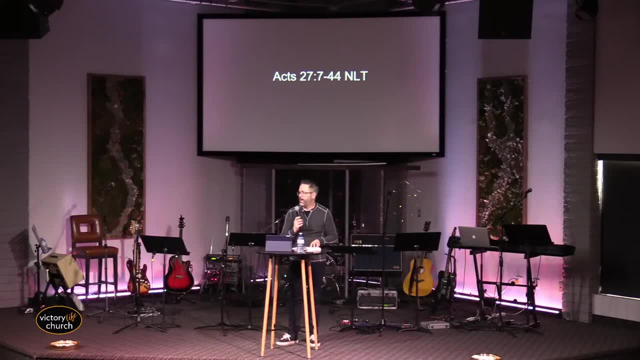 for you will surely stand trial before Caesar. Yay, Don't worry, Paul, You won't come to see me tomorrow. You still got to go stand trial. Awesome, Thanks, God. What's more, God in his goodness, has granted safety. 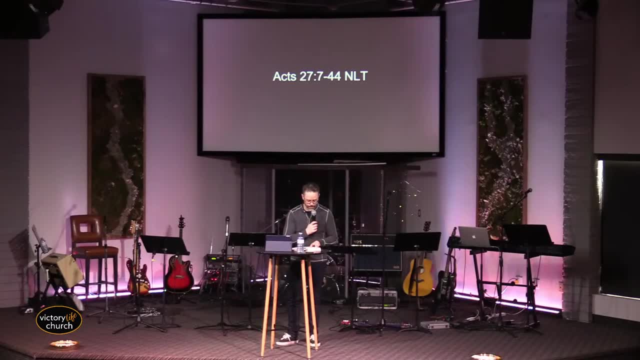 to everyone sailing with you. So take courage, for I believe God, And it will be just as he said. Paul is saying here. it may not turn out how you think, but if God is in control, we can trust him. He will give us new direction. 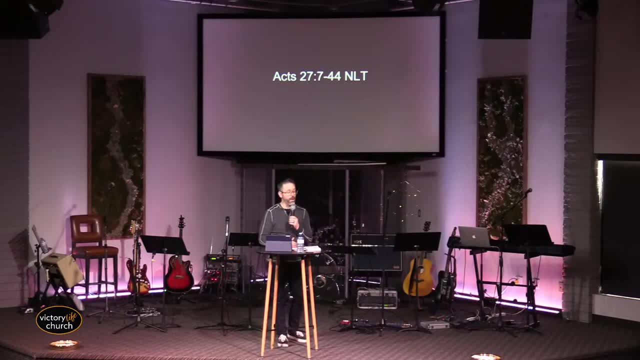 He will show us how to press through. He'll give us a choice: follow God or follow our own understanding. Proverbs 3 and 5 says: Trust in the Lord with all your heart and do not depend on your own understanding. He goes on. 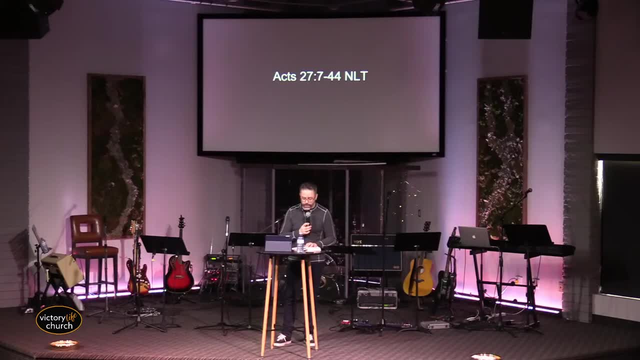 He says Verse 26,. But we will be shipwrecked on an island, Yeehaw. About midnight on the 14th night of the storm, as we were being driven across the Sea of Adria, the sailors sensed land was near. 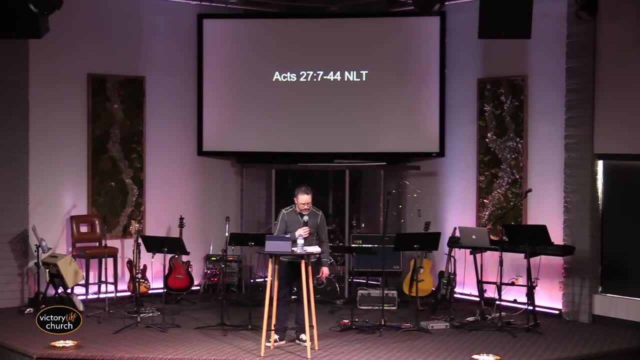 They dropped a weighted line and found that the water was 120 feet deep. But a little later they measured again and found it was only 90 feet deep. At this rate, they were afraid we would soon be driven against the rocks along the shore. 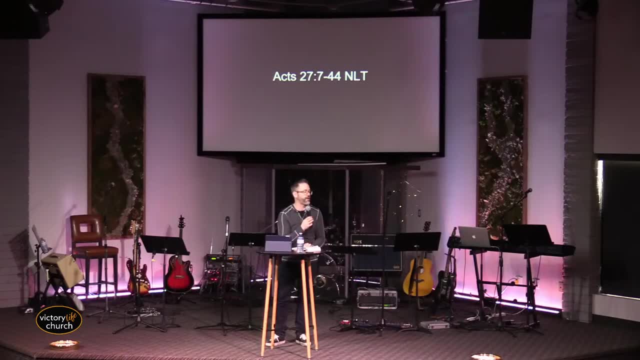 So they threw out four anchors from the back of the ship and prayed for daylight. Then the sailors tried to abandon it. They abandoned the ship, They lowered the lifeboat as though they were going out to put out anchors from the front of the ship. 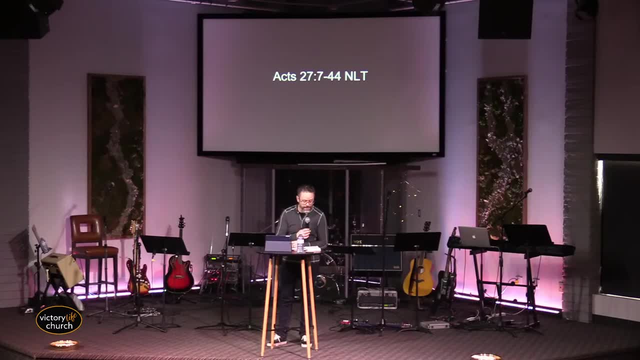 But Paul said to the commanding officer and the soldiers: You will all die unless the sailors stay on board. Don't try to abandon God, Don't try to abandon Holy Spirit. It may look difficult, It may look impossible, But stick with the Spirit. 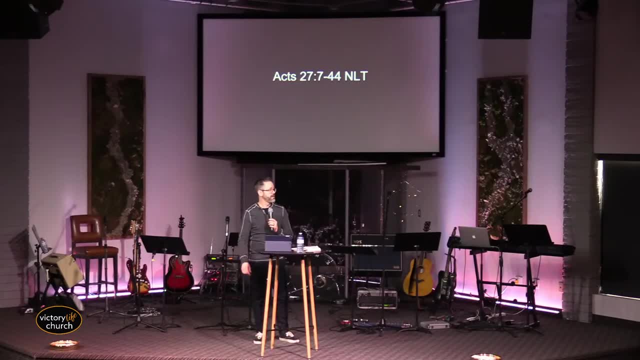 Amen. With God, all things are possible. He goes on in verse 32.. So the soldiers cut the ropes to the lifeboat and let it drift away. And in verse 33, it says: Just as day was dawning, Paul urged everyone to eat. 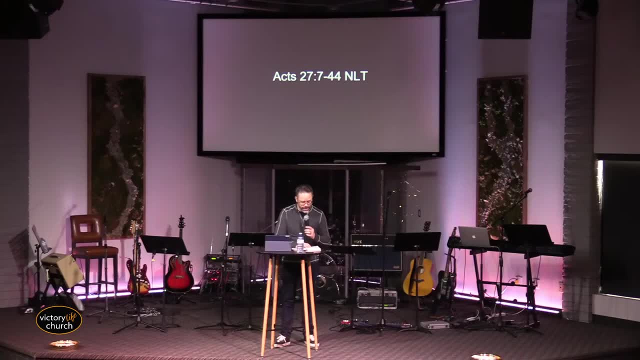 You've been so worried that you haven't touched food for two weeks, he said. Worry will cause us to forget to feed ourselves the bread of life. Generally, if you've abandoned reading your word, you've abandoned praying, you've abandoned attending church, 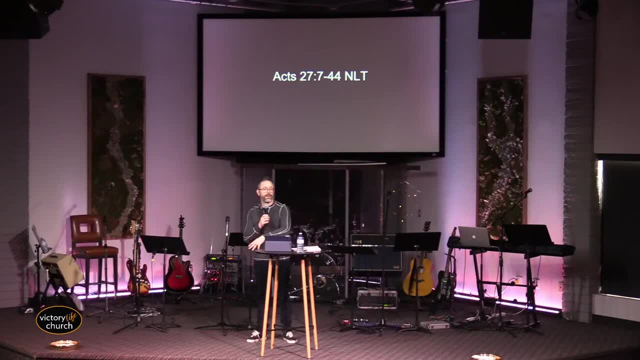 you've abandoned fellowshipping with other believers during your storm. that's a pretty good sign. you're using your own strength. You're trying to do it in your own strength When you abandon feeding yourself because of the worry we've got to keep going. 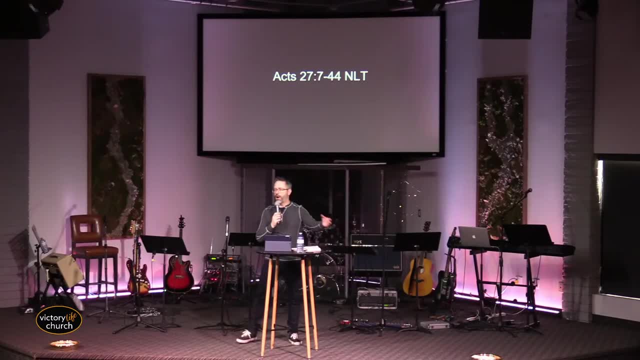 We've got to continue with God. Keep asking, seeking, knocking. The answers are here. This word is alive. It will speak to you and answer for your situation. Verses 39 to 43,. it says When morning dawned. 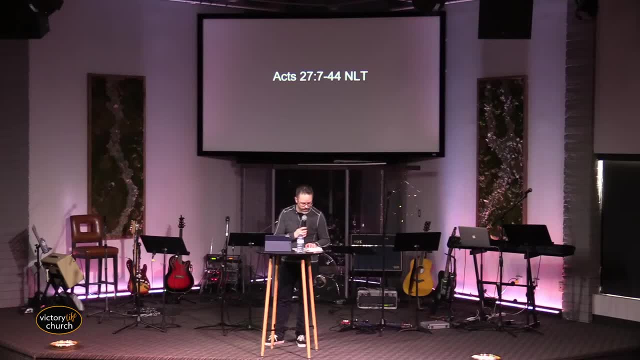 they didn't recognize the coastline, but they saw a bay with a beach and wondered if they could get to shore by running the ship aground. So they cut off the anchors and left them in the sea. Then they lowered the rudders. 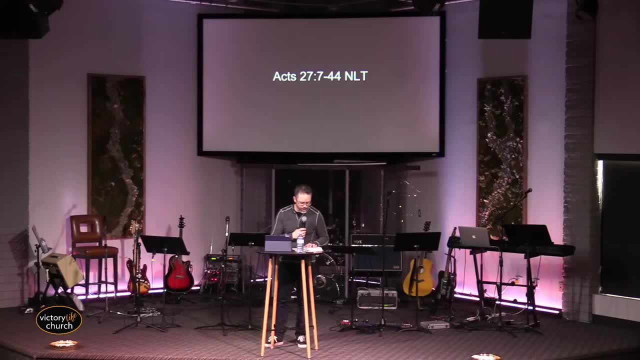 raised the foresail and headed toward the shore, But they hit a shoal and ran the ship aground too soon. The bow of the ship stuck fast while the stern was repeatedly smashed by the force of the waves and began to break apart. 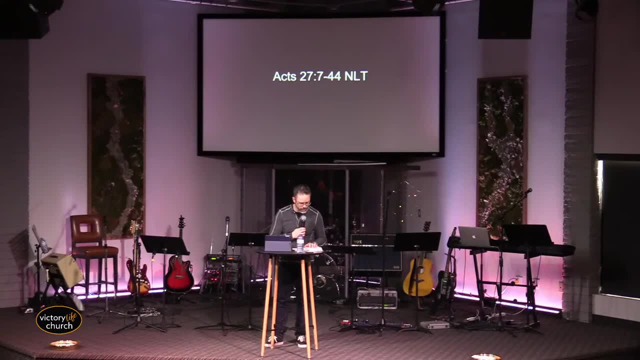 The soldiers ran wanted to kill the prisoners to make sure they didn't swim ashore and escape. But the commanding officers wanted to spare Paul, so he didn't let them carry out their plan. Then he ordered all who could swim to jump overboard first. 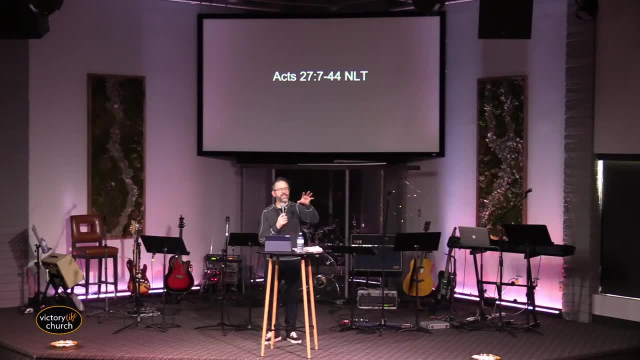 and make for land. Even when you see a light at the end of the tunnel, they saw it- Land ahead. There may be something that's come along to try and derail or sink you, But those who can swim, and even those who not yet can swim, 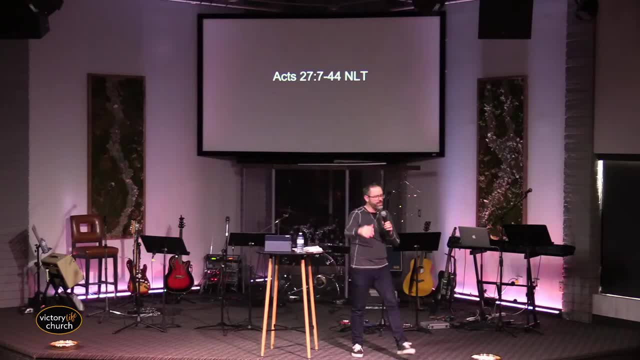 even those who maybe, you know, maybe there's those of us who are like, yeah, I fully trust in the Lord and you jump in the water to swim, And maybe there's those of us standing on the boat going. I don't know totally yet. 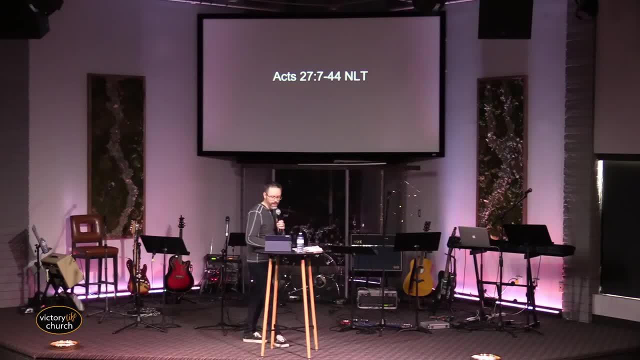 Guess what? That's okay, Jump in. Why, When we trust the Lord, it says this: 44. The others, he said. then he ordered all who could swim to jump overboard first to make for land The others. 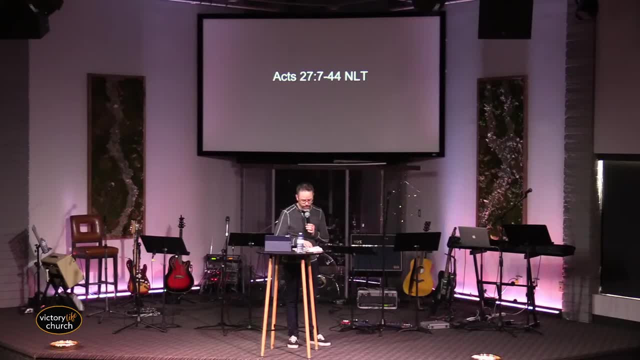 so those that couldn't swim held on to planks or debris from the broken ship. so everyone escaped safely to shore. Even if you're right now, you're struggling in the faith, you're struggling to trust, jump in the water God will provide from the brokenness. 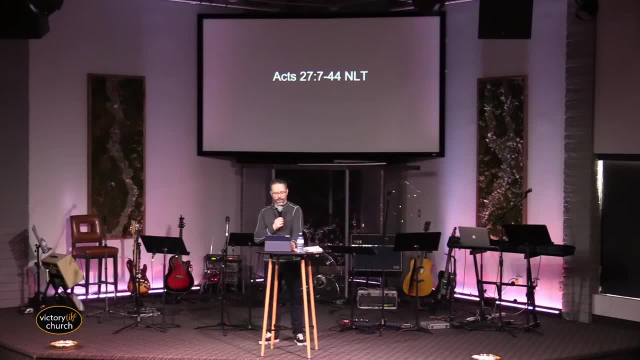 something to grab onto to get you to shore. Now are there consequences to not following God's instructions? Mm-hmm, The boat and its contents were completely lost in the storm, And it may seem like the sailors lost everything that was important. 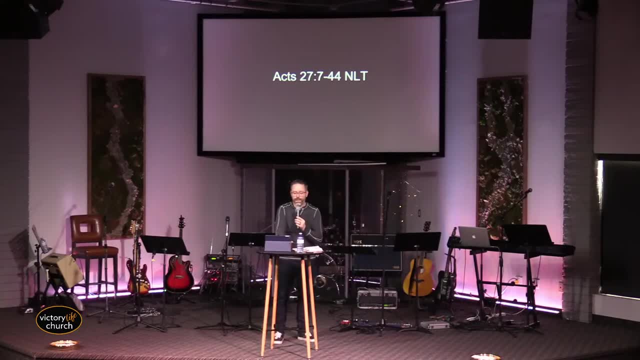 It may not be your destination, But they still had their lives. Give God glory. Share him where you're at. You know wherever you arrive, even if it's not where you thought you were gonna be. give God glory. Share him in that situation. 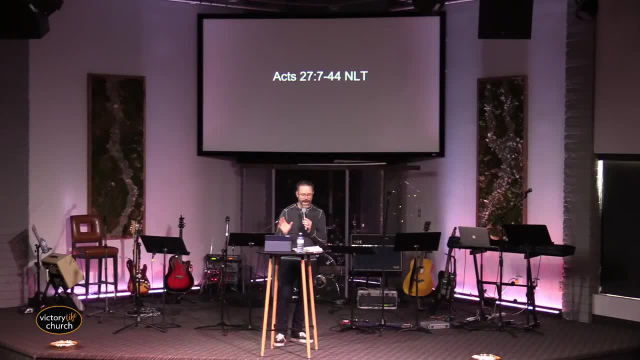 Because I love that: Do everything you're called to do. because I love this next part in Acts 28,, verses 7.. Acts 28,, verse 7, it says Nice name- The chief official of the island. he welcomed us and treated us kindly. 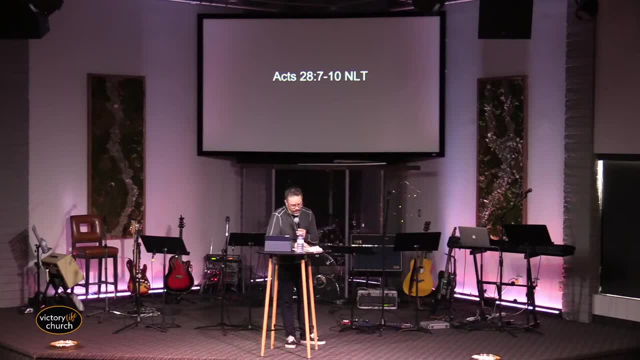 for three days. As it happened, his father was ill with fever and dysentery. Paul went in and prayed for him and, laying his hands on him, he healed him. Then all the other sick people on the island came and were healed. 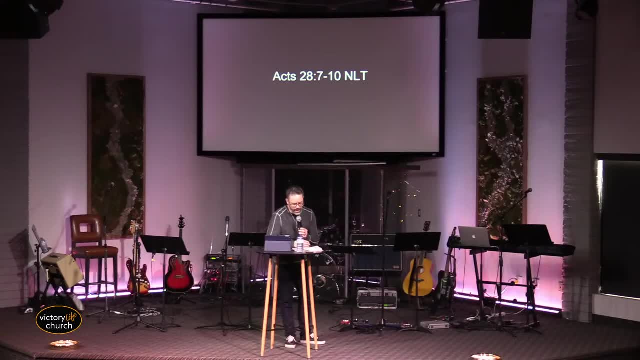 As a result, we were showered with honors And when the time came to sail, people supplied us with everything, everything we would need for the trip Man. you wanna underline that portion? Paul came, He's like you know what. 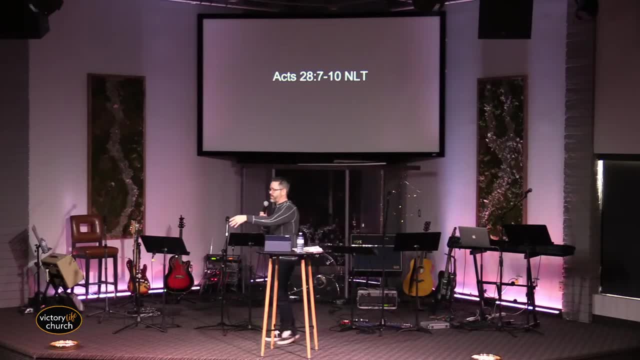 This isn't where we planned to be. This isn't where we were supposed to be. Some of the poor decisions got us here, but God brought us here alive. We may have lost the ship and the contents, but God brought us here alive, amen. 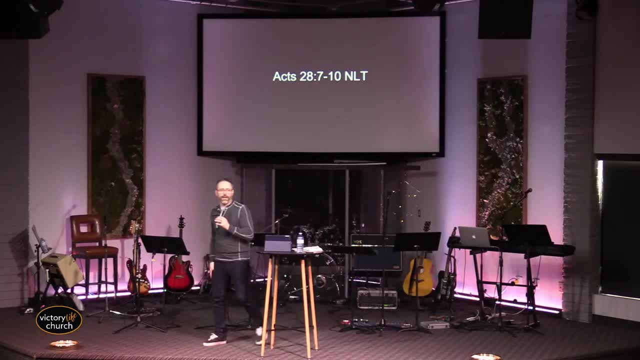 You might be sitting here today and you think I've lost the ship and I've lost the contents. Are you breathing? God brought you here alive. God has brought you through this situation alive. You might feel your ship is sinking. You know what? 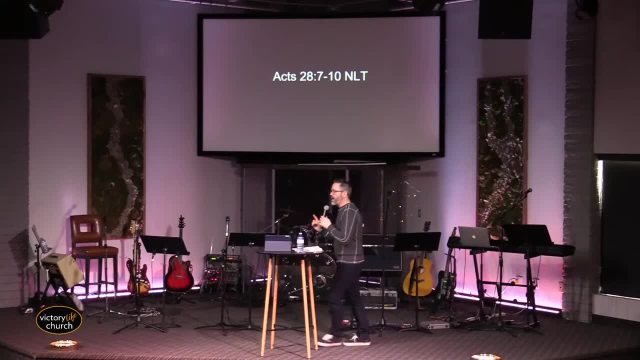 Sometimes letters sink. God's bringing you through alive and continue to seek him. continue to do God. Paul shared the gospel, He showed and used his faith And, as a result, when it came time to set sail again to their destination. 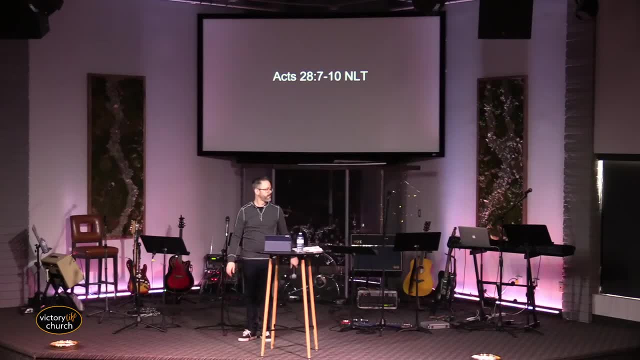 they were supplied with everything they'd need for the trip. That is a mic drop When it comes time, when it comes time for God to get you back on path to your promised land, if you are faithful in the time where you're not where you thought you would be. 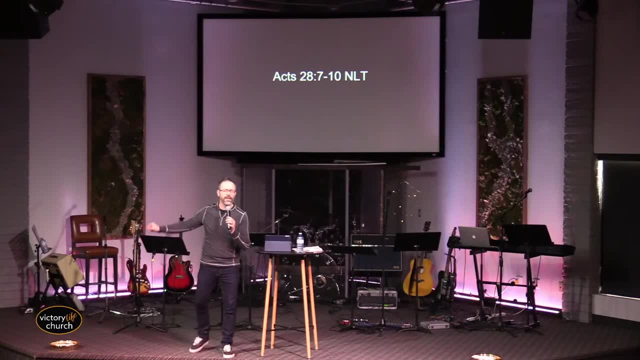 if you are faithful and you continue, and you continue to seek him, you continue to glorify him, you continue to do what he called us to do and to go all the world. preach the gospel, make disciples. you continue to share. You may not be where you thought you'd be. 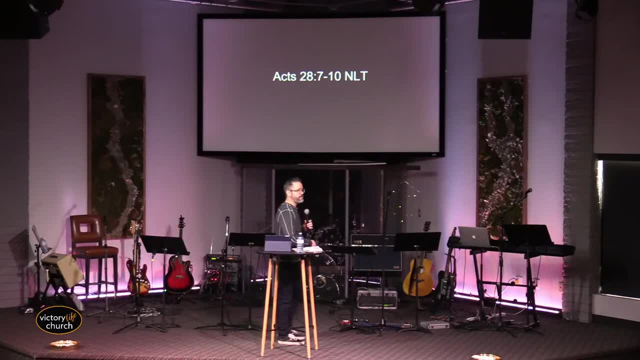 but, thank God, you're not where you used to be. amen, And then he will equip you and he will give you and supply you everything you need to make this world a better place. Make that trip to the promised land When you set your heart to share the gospel. 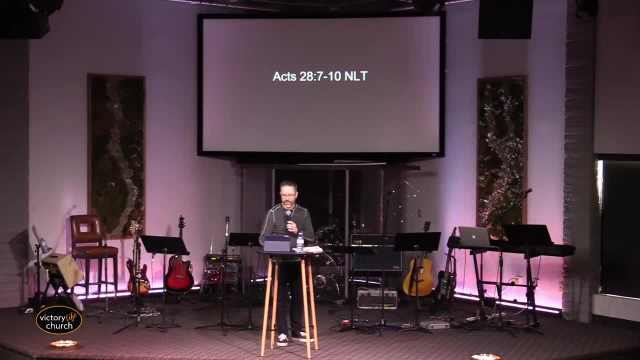 live the gospel in all circumstances. wherever you're at in life, even if it's not where you expected, God will supply all your needs according to his riches and glory, through Christ Jesus, amen. Today's takeaway is this: We need to exercise listening to the Holy Spirit. 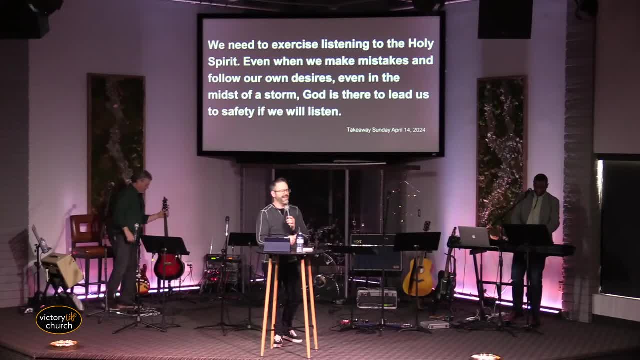 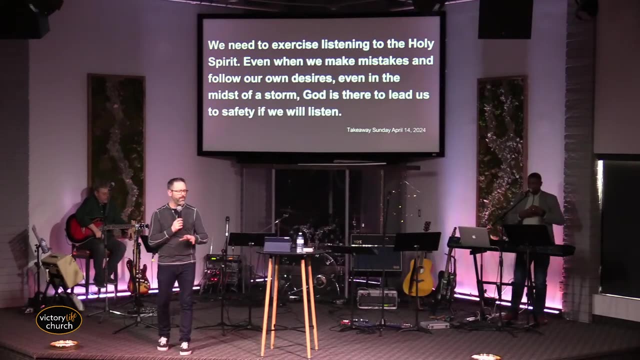 Even when we make mistakes and follow our own desires, even in the midst of the storm, God is there to lead us to safety, if we will listen. amen, Amen, That's Holy Spirit. The Bible, the New Testament, talks all about being led by the Spirit and not by the flesh. 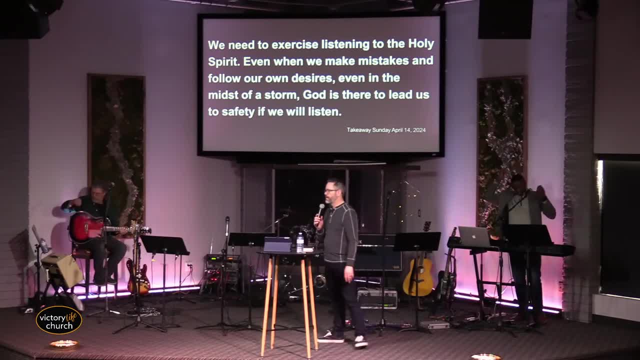 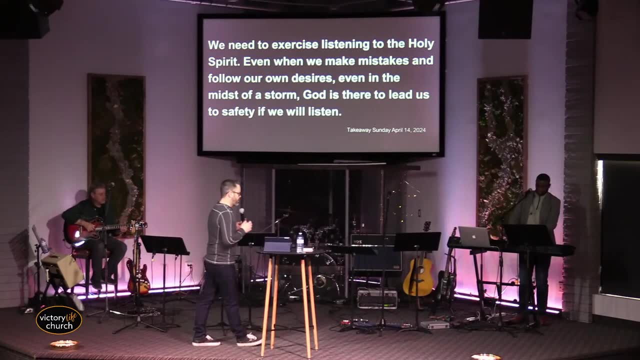 Not being led by our own desires, but being led by the Spirit. Today, if that's you. you know we've talked times and before about the baptism of the Holy Spirit. You know, when we accept Jesus as Lord, the Spirit of God comes to live inside us. 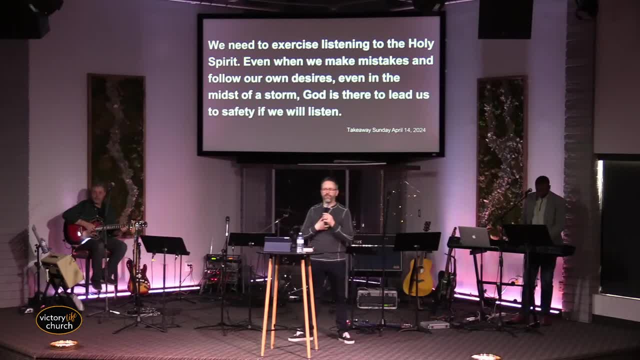 comes to take up residence without ever intending to leave. But then we've also talked about the baptism of the Holy Spirit. when the Holy Spirit comes upon you and endues you with power from on high and gives us even that next level power and that next level ability to listen to him. 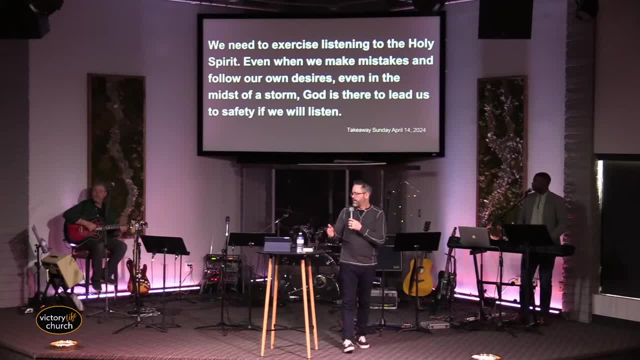 and lead us and guide us. And Luke says that if we, as fathers, would not give our kids serpents, we would not give them serpents When they ask for bread and bad things when they ask for good things. how much more will God give us the Holy Spirit? 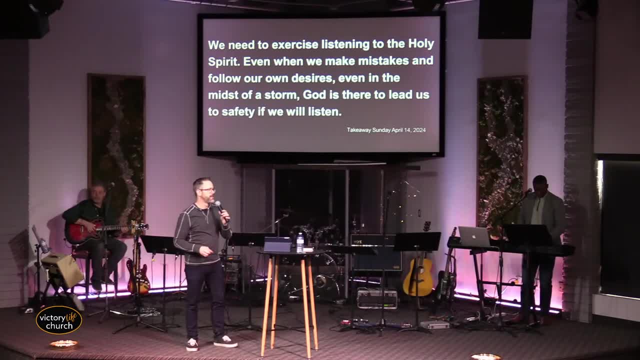 How much more will God give the Holy Spirit to those who ask him- And that's something I want to encourage you to really pray about- If you haven't received the baptism of the Holy Spirit this time and you're like I don't know? 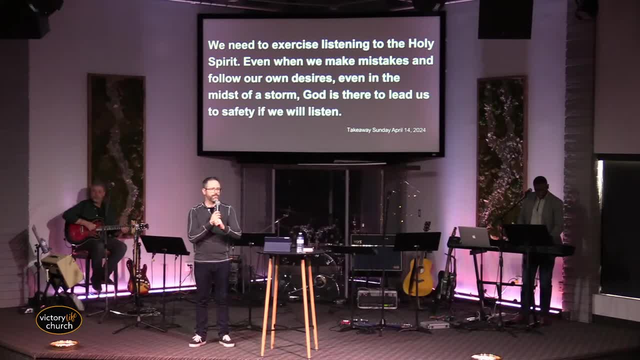 the thing is: how bad do you want it? That's the thing. You could come up for prayer a hundred times believing that if one of the pastors lays hands on you and prays for you, and prays for you, the baptism of the Holy Spirit is going to fall. 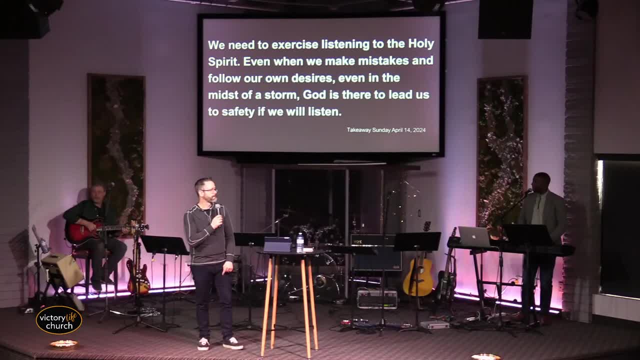 It's: how much do you want it? And when we're like God, I want that, I want it. God, I believe your word says that if I ask, I will receive the Holy Spirit from you When we get to that place of the desire in our heart. 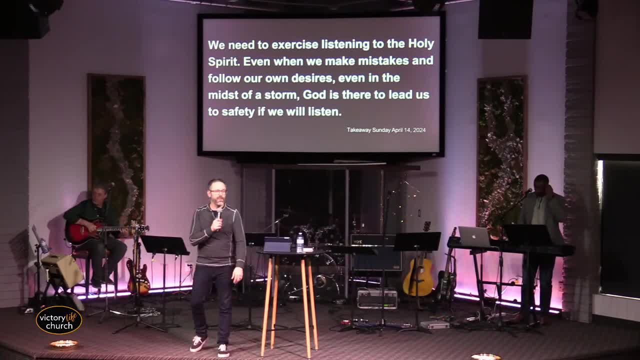 that's when you come and see one of the pastors. I mean, I've seen people that they're just praying and believing for it and boom, Holy Spirit falls. You read accounts in the book of Acts. Peter came, was preaching the gospel. 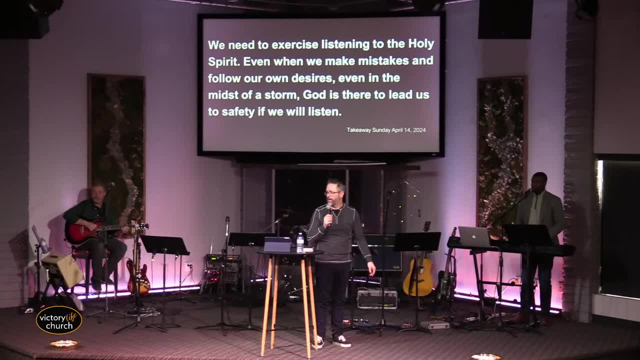 and all of a sudden they started speaking, Speaking in tongues, praying in tongues, live there, And sometimes it's now. it's like I want to, I want this, And then somebody can pray with you, Somebody who has already received the baptism. 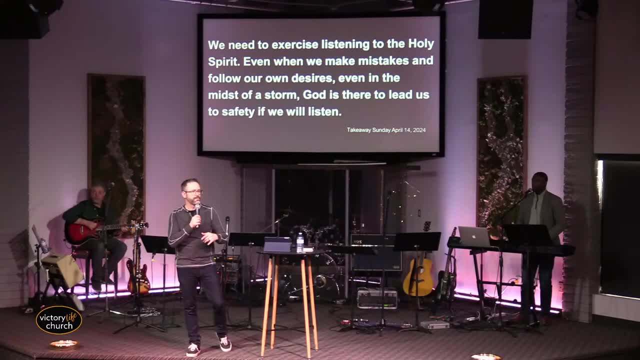 of the Holy Spirit, pray with you And then it comes. So today, if you're here today and that's something you're like God, I want that, I want this, I want this. Begin to pray into it. 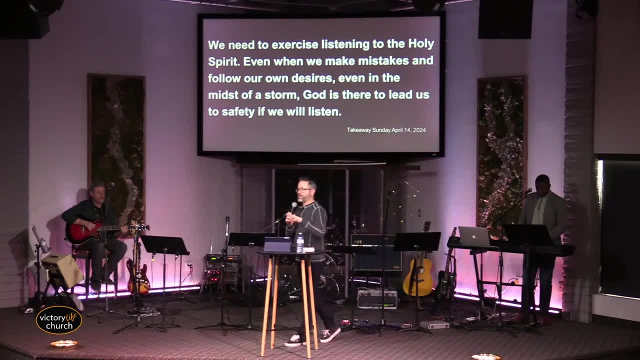 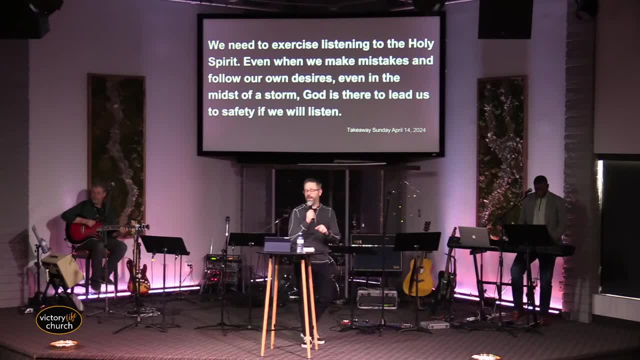 Begin to seek it, Because God is faithful And we will have an opportunity. during this series. We will pray, But today I wanted to encourage you just to continue to seek it. Continue to seek it. Get it into that place in your heart. 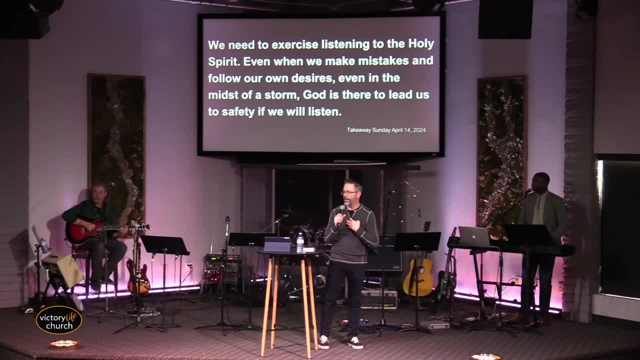 that hunger So great, Amen, That hunger is so great. Watch, it might even happen while you're sitting at home and you're in your word and all of a sudden you'll be like Lord, I just want a rabba shakat, a rabba sado. 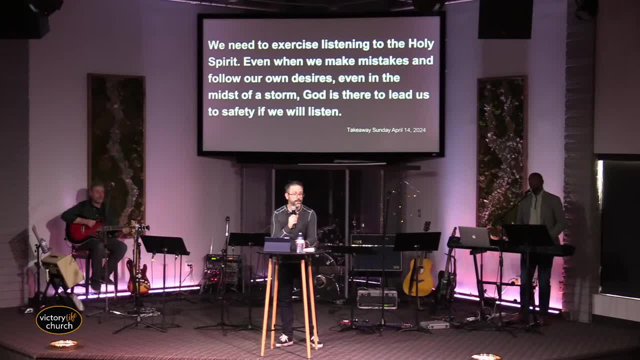 Who is that? That's Holy Spirit coming in, Shutting your brain off And allowing you to pray as perfect will: Amen. Now, if you're here and you're like I don't even know Jesus, I just need to know this Jesus that comes in. 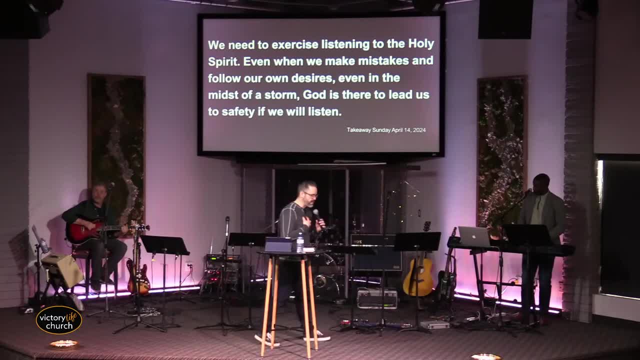 and He'll lead me and guide me. You know what? It's very simple. Romans 8, Romans 10 says: Confess with your mouth that Jesus is Lord. Believe in your heart that God raised Him from the dead. That's where we begin that relationship with Him. 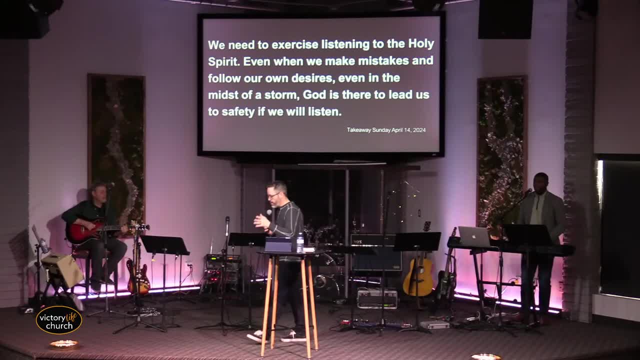 If that's you here today or you watching online, I would be remiss not to invite you to pray a prayer with us. We'll pray it along with you, With every head bowed and every eye closed. we say: Dear Jesus, today I declare that You are Lord. 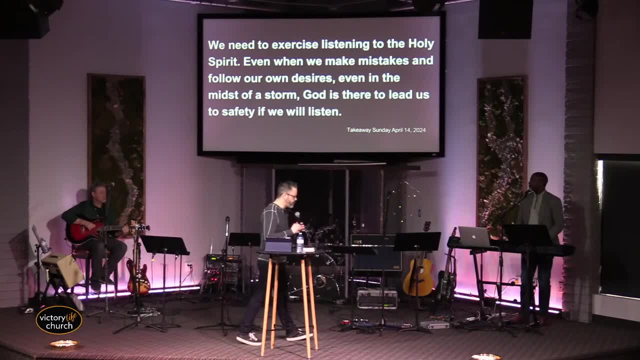 You are Lord of my life And that God raised You from the dead, I believe. Lord, thank You for Your forgiveness of my sins and my mistakes. Thank You for giving me a fresh new start at this life, Despite all my mistakes. 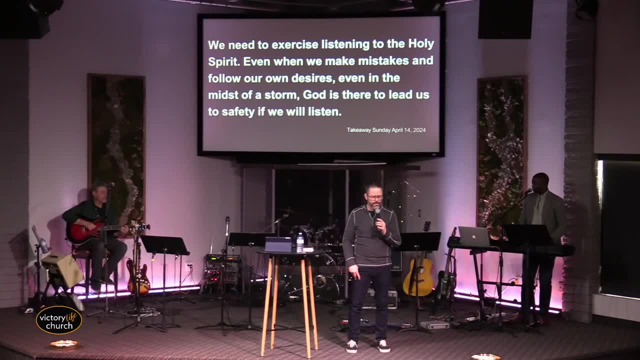 I may not be where I want to be, but with You You will lead me on the path of life. Please help me to follow You In Jesus' name, Amen, Amen. If you prayed that prayer for the first time today, 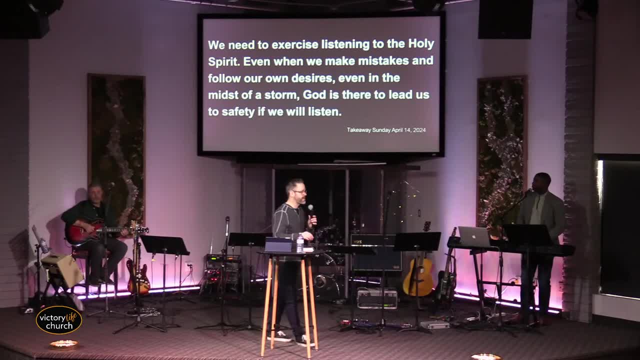 thank you. That is awesome. We're excited because the heavens rejoice when one more person recognizes Jesus as Lord. Welcome to the family. Let us know. Fill out a Connect card. If you're watching online, go to our website. Go to our contact page. 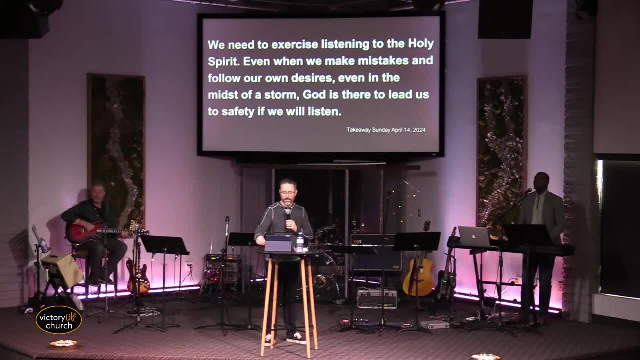 Let us know. We're excited about that. What's next? Well, come back next week. Amen. Continue to be a part of the body of Christ. Continue to feed yourself, Continue to be a part of this. Connect with somebody this week. 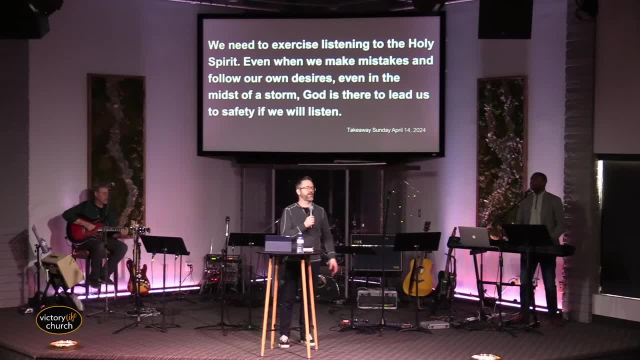 If you've been praying for the Holy Spirit, you're believing for the Holy Spirit. you know somebody that's baptized in the Holy Spirit. call them up and say: Hey, Come pray with me, Read your Bible daily. You got a whole section of the book of Acts to go through. 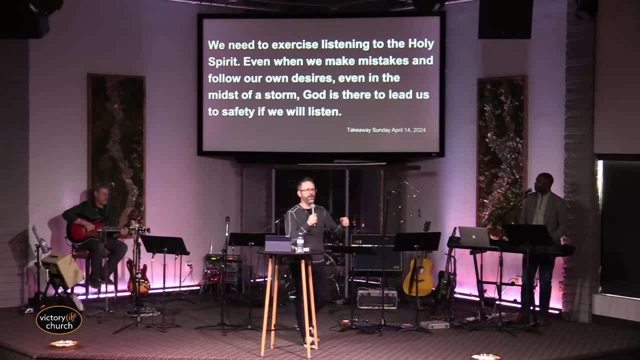 Read that story about the ship and read and apply it and see where you can go. Oh, that's my life, This is the situation, and we can begin to see, and God shines lights on things and illuminates areas where we go. Whoa, that's so cool. 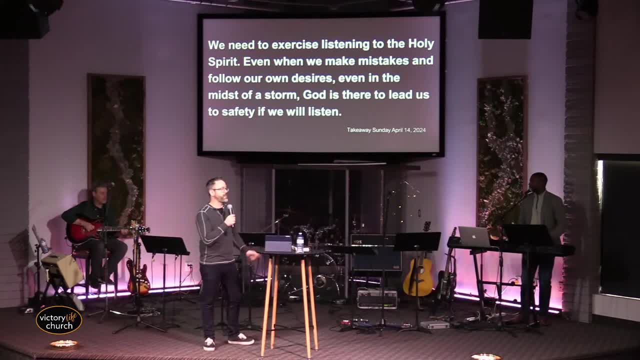 Now I know to go this way. Amen, That's how Holy Spirit speaks to us. Next is to find a place to get involved. Be a part of the body of Christ, Be a part of what God's doing, Be a part of the movement. 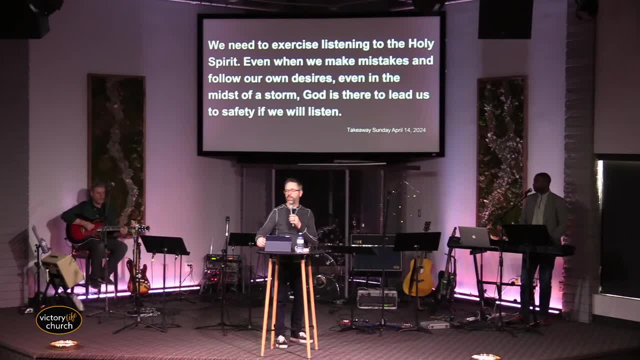 And, lastly, invite somebody to come back with you next week, because that's the gospel mission: To reach people. To reach people, Those that may have heard but have never accepted the good news yet that Jesus died for them, He rose again for them. 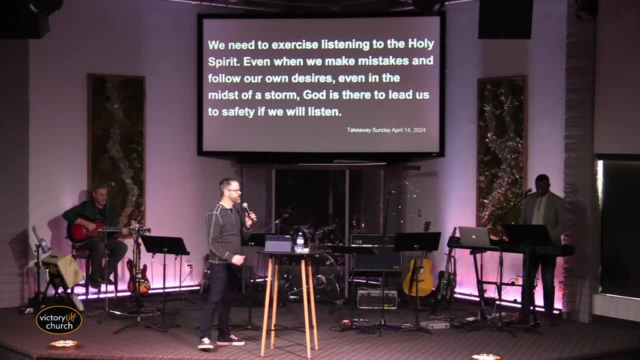 Amen, Amen. The victory on the cross and victory when He rose again. Lord, I just thank you for that, Lord, I just thank you for today, and I thank you for each and every one here. I thank you, Lord, that you would give us. 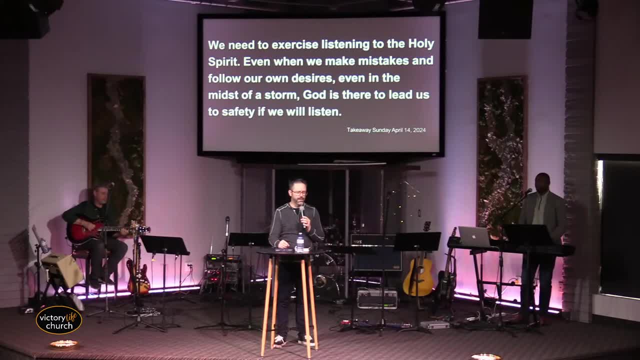 ears to hear and eyes to see Holy Spirit in our lives. An acute sense of hearing to hear that still small voice to lead us and guide us into the goodness that you have for us. Lead us and guide us into the promises you have. Lead us and guide us into life abundant. 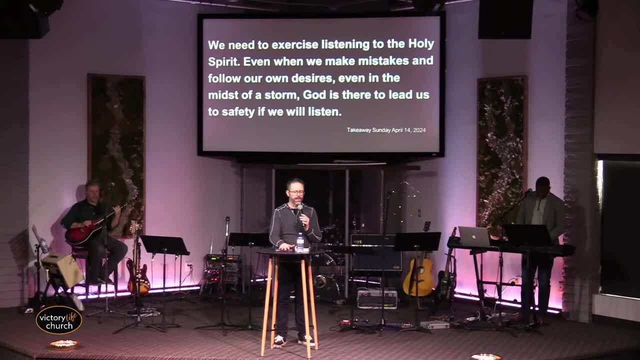 that Jesus said we would have in Him. Amen. I thank you for that today In Jesus' name. Amen, Amen. God bless you all. I pray you have a wonderful week. Don't forget about Wednesday morning prayer, 6 am, if you're able to join us. God bless you all.